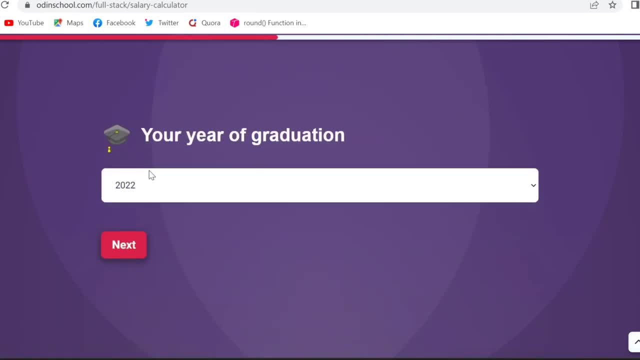 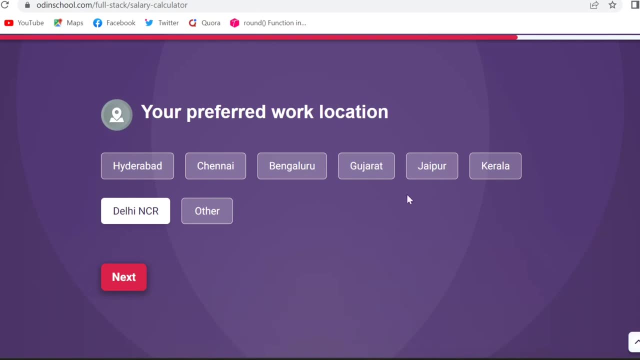 link, this type of page will be opened And you just have to fill your name, your educational and professional details, highest qualification, year of graduation, work experience, job role you are looking for. preferred work location. work location, mail id, phone number and you. 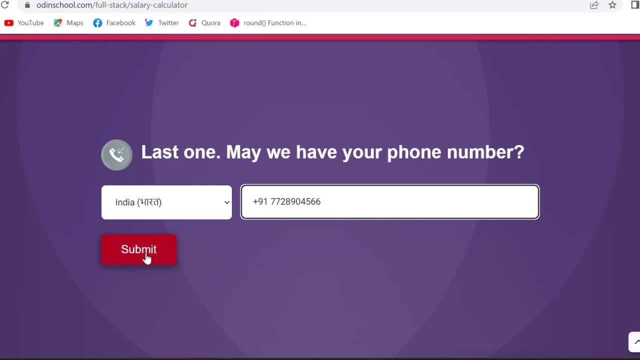 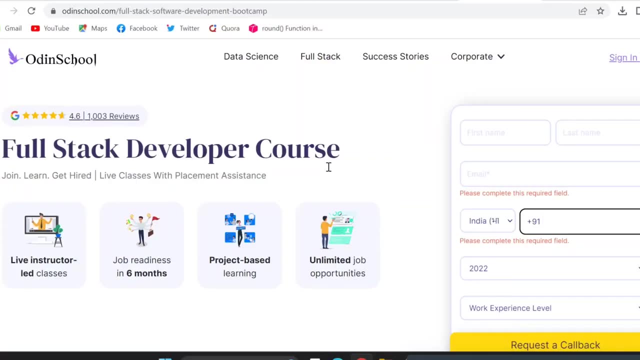 just have to submit And then it will show you how much you could earn per annum. This is just a estimate According to you are given answer. so if you are interested in full-stack software development, then odin school is conducting a six-month full-stack software development bootcamp, and this bootcamp is perfect. 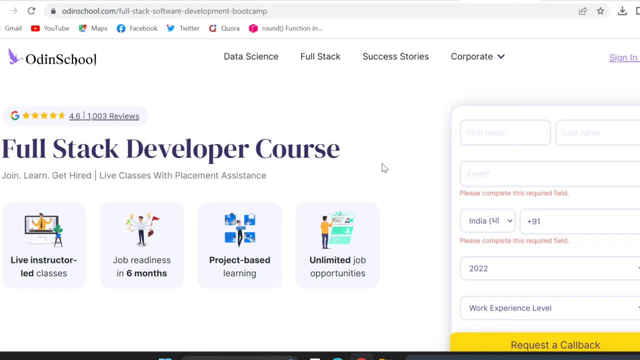 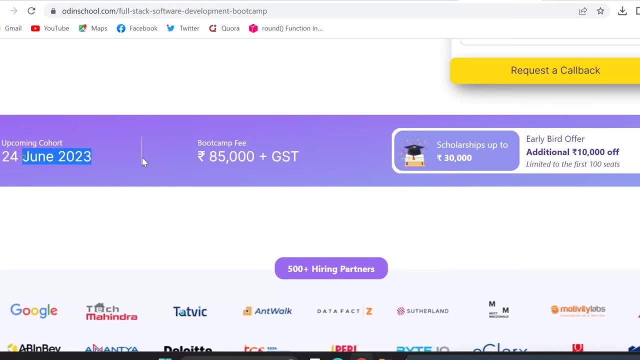 for anyone who wants to access industry-aligned education at a reasonable price. as you can see the detail- the next cohort would be started from 24th of june- the free detail you can see as well- as you will get a scholarship up to rupees 30 000 and there is an early bird offer in which you 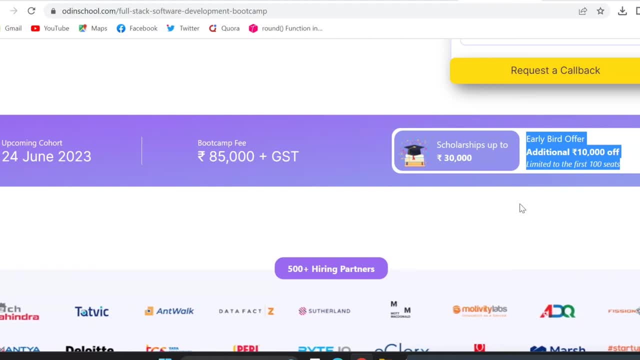 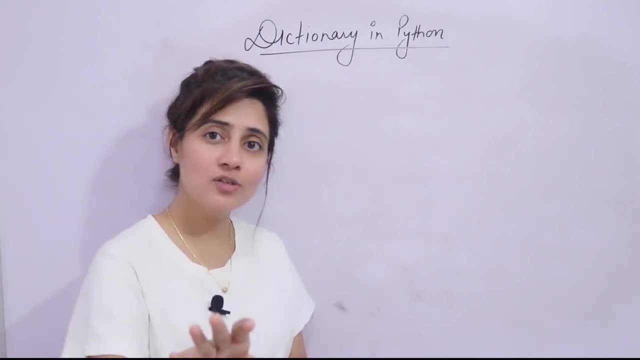 will get 10 000 additional discount and no post tmi option is also available. that's not it. it comes with two one placement records and 360 degree placement assistance. don't just go with my words. you can check out their success stories. you can check out on their website many success stories. 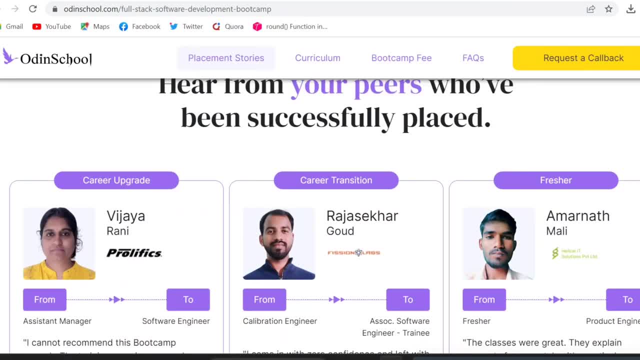 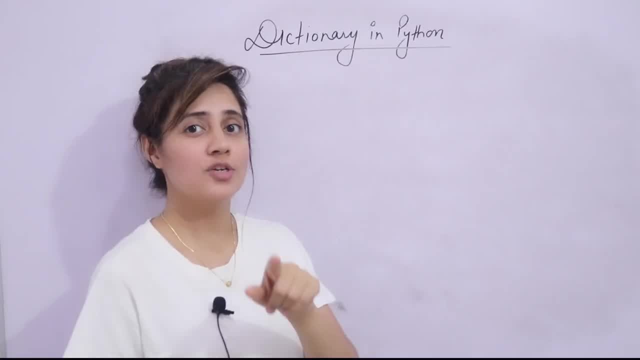 you will get of their students because they are having 500 plus hiring partners like google, tcs, infosys, capgemini, deloitte, many more top tech companies. so if you want to start your career in full stacks of your development field, join odin school today. how to apply for this bootcamp. 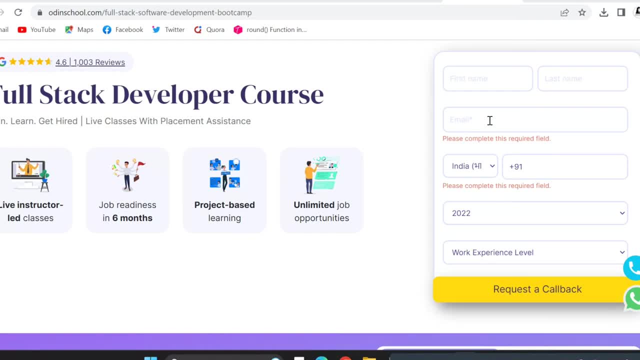 you can just click on the link that i'll put in the description of the description box of this video. once you click, this type of page will be opened. you just have to fill out this detail, the basic detail, and you can request a callback. now code in school team is going to call you back. 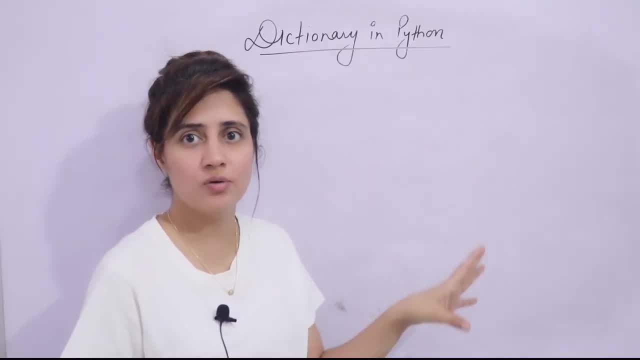 within one or two days, whatever doubt you have, you can ask your doubt, clear your doubts and then pay the fee and then enroll in the course. so all the relevant links and details you will find in the description box of this video you can go and check out. now let's see. okay, let's take a real example. 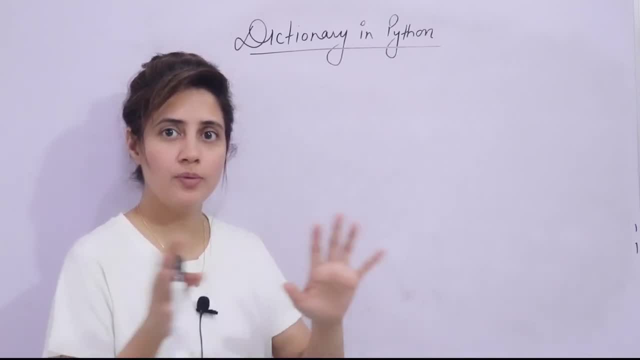 like in our home also we are having dictionaries. if you don't know meaning of anything, we just use to search the that meaning of that word in dictionary. okay, nowadays we just search on google the meaning of that word, but we used to have dictionaries once. right now, if suppose you want to search meaning of beautiful, so we will search. 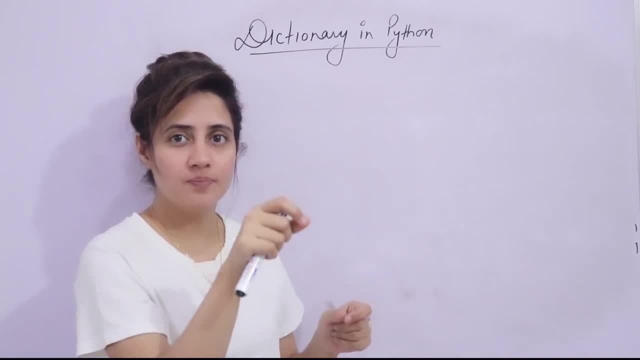 like from index, like from where the letters of b would be started, then b, then b e, then ultimately, we will search: where is this that beautiful? after finding that word beautiful, we will see the meaning of that beautiful, that word right, like this. so how the this data is to be stored in? 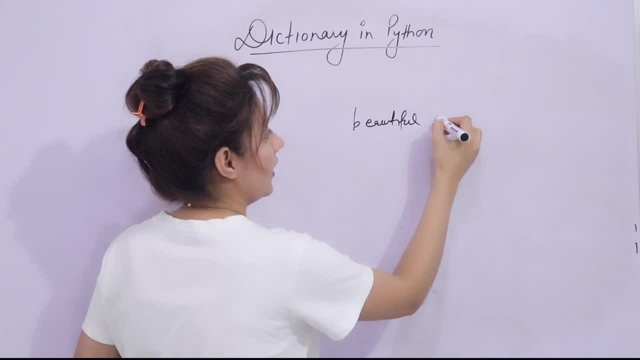 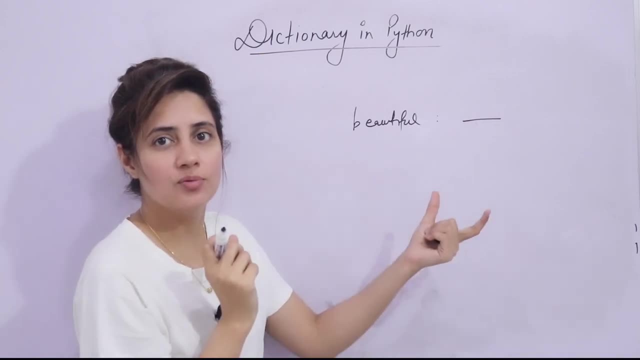 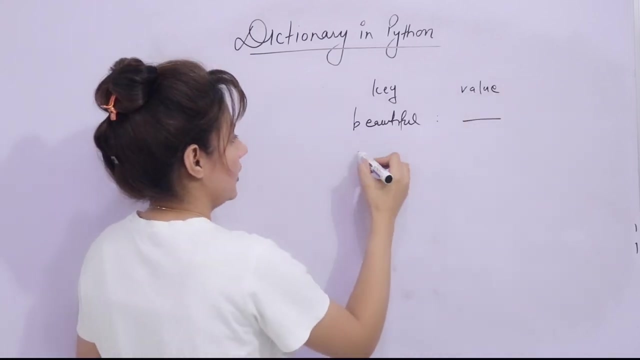 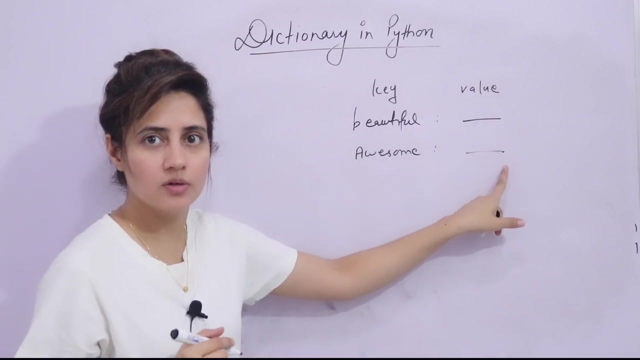 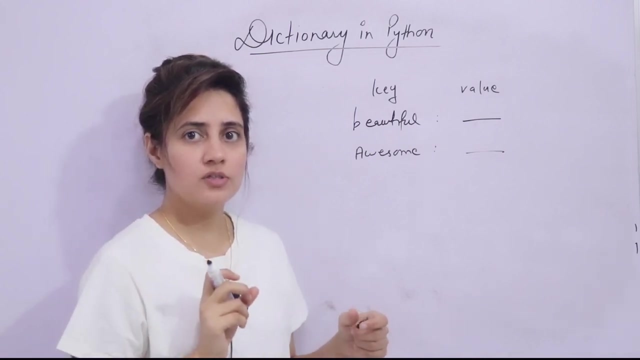 dictionary like first beautiful and then meaning. meaning of this right means in a form of key and value: this is key and this is value. another word like awesome: this is key, and here we have meaning of that word. like this: if suppose you want to search in a dictionary, you want to search phone number of anyone, so we'll search first. 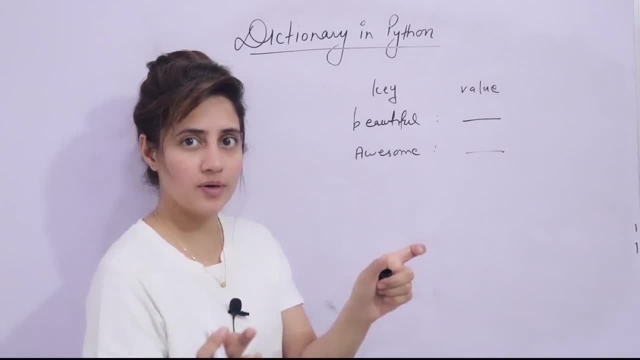 like the name jenny, okay, jenny, and then we will get the phone number. ultimately, we'll retrieve the phone number. so here jenny is the key and phone number is the value of jenny. so key and value pair. in real life we used to deal with these type of data arrangements. 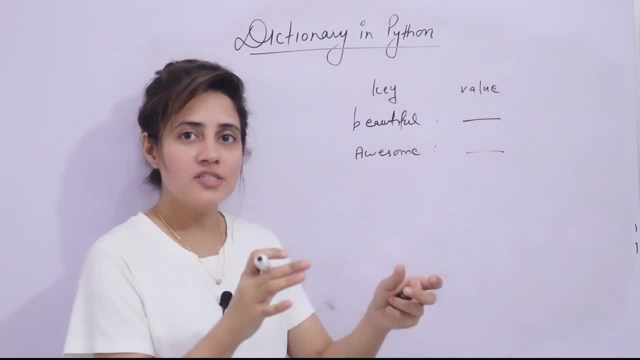 every day right now. this type of data arrangements we can also imitate in programming language, in python, in the in program. if we use to store this type of data arrangement in a key and value pair, then we have something and name is same. that is dictionary. we have a data structure or we can say a built-in data type. we have to store collection. 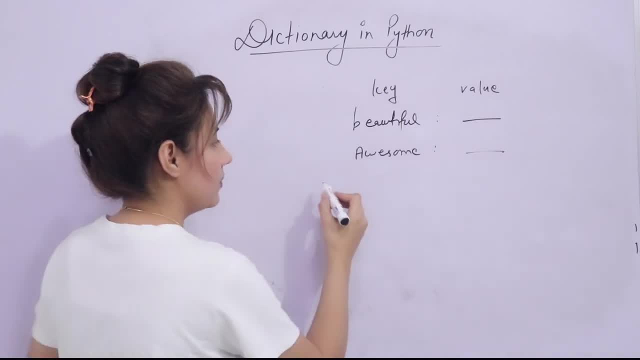 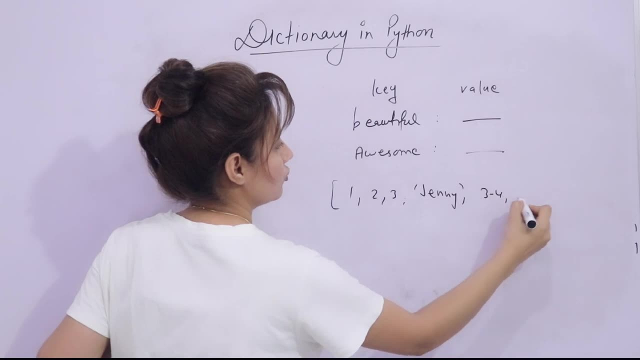 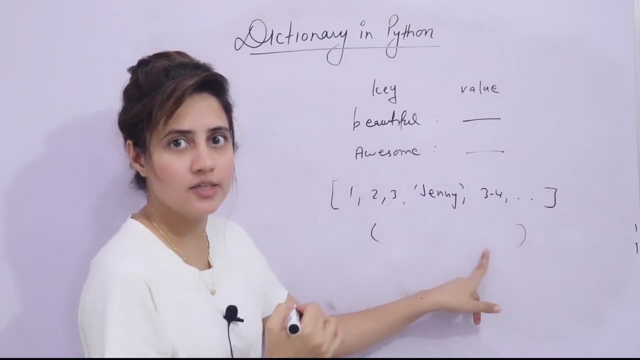 of data. that is dictionary. see in a list what we store. something like this: like one, two, three or like string also we can store, or any float value. we can store something like this: list of items in a set. also something like this: any set of items and tuples also, but in form. 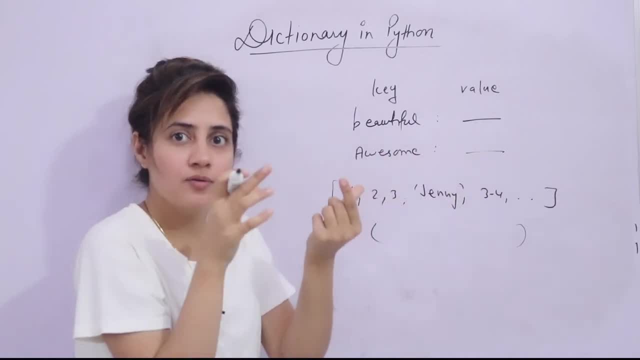 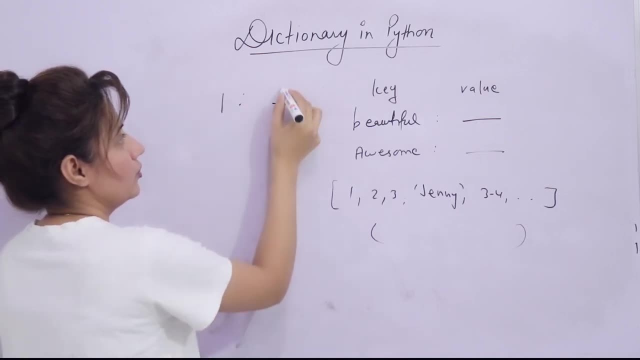 of pair, if you want to store the key and value pair for that particular thing. we are having dictionary like I am going to store roll number of student and then name of that student, like jenny, roll number of the student. then if we write down in register maybe something, 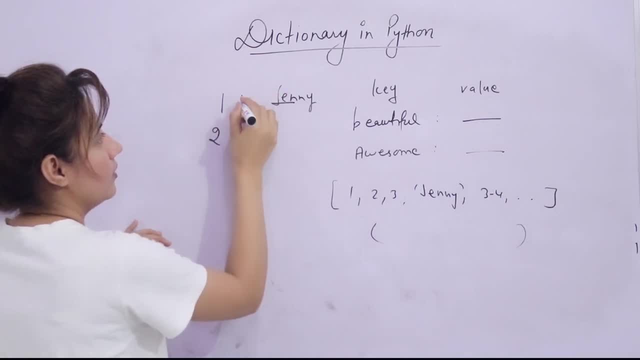 like this: we can write 1 and dash, or 1 equal to or 1 colon, something like this we write. but here we have a proper syntax. that also I will tell you. in programming 2 suppose ram 3, anyone right? so here also we are having key and value pair, if you want to find out. 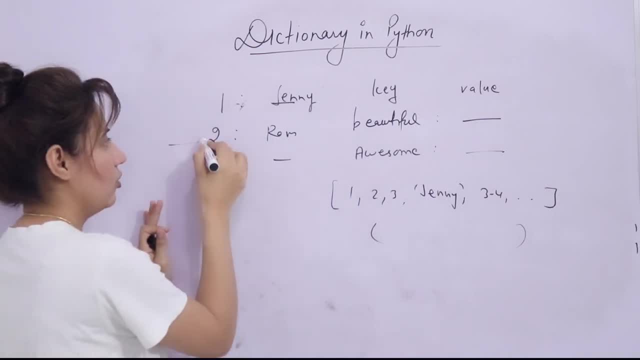 name of any student, just if you know the roll number. just look for the roll number of that student and then you can store it And you will get the name of that student. roll number 2: what is the name? just look after in your register what is the, where is the roll number 2, and then you will get. 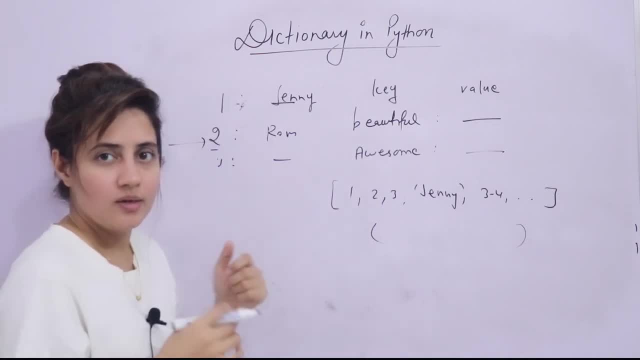 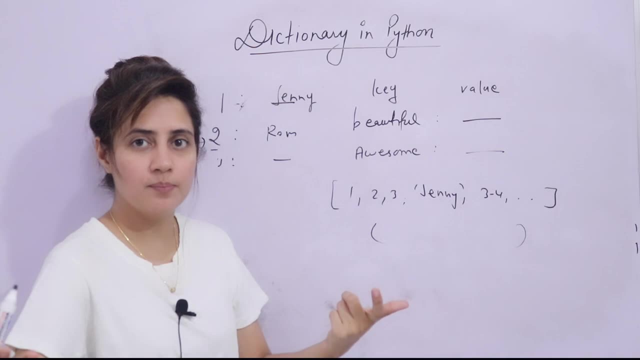 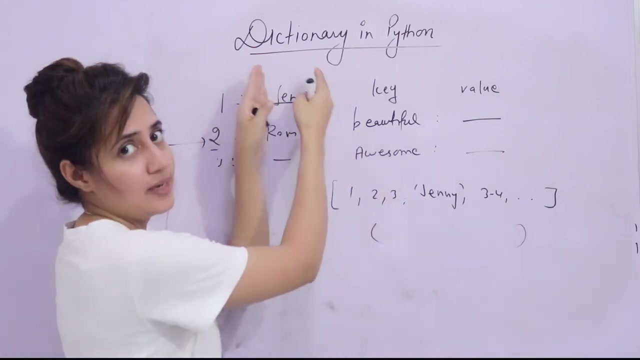 the name. so this is key. this is value right Suppose in a company: employee id and employee name, or maybe employee name and salary of that employee, like this type of data arrangement. if you need, then we use this type of built in data type that is dictionary in python right. 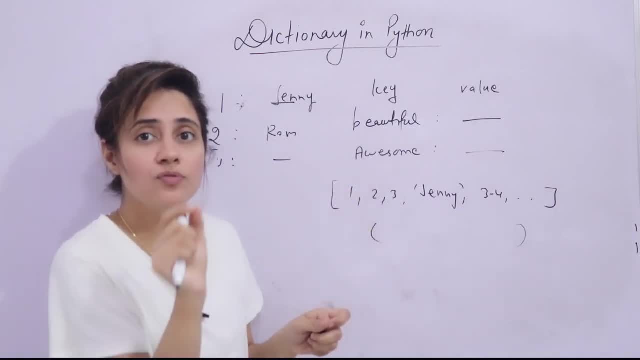 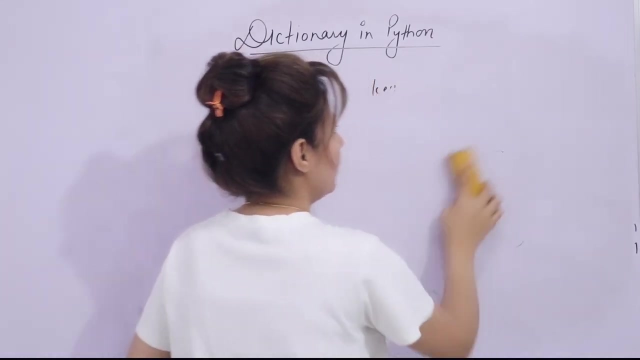 So it is used to store collections, So collection of data in the form of key value pair, key value pairs. I hope you got what is dictionary and what is simple. you know definition or meaning of dictionary and why we use which kind of data. if you want to store and see, this is very helpful. why so? 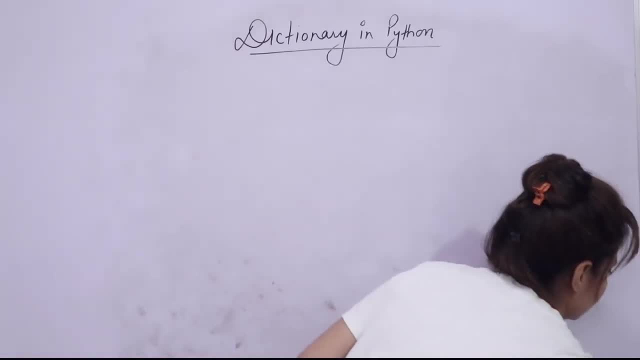 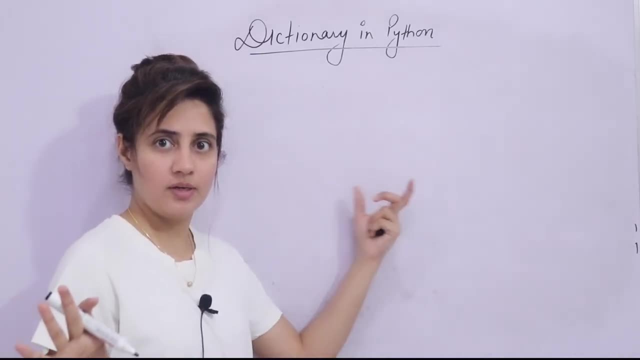 I have already told you because, using dictionaries, we can imitate, or you know, that real world data arrangement in programming, Where, Where each key is associated with a particular value, right, That type of thing, that type of scenario, data arrangement, we can imitate or we can. 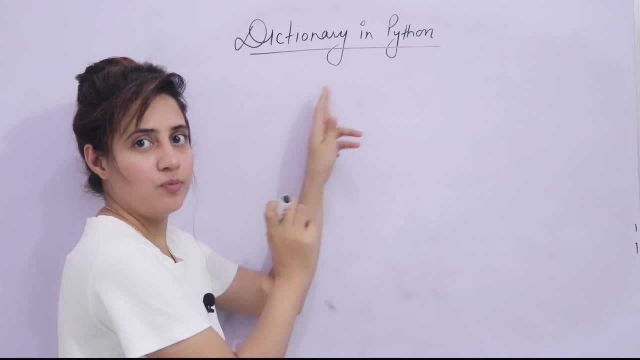 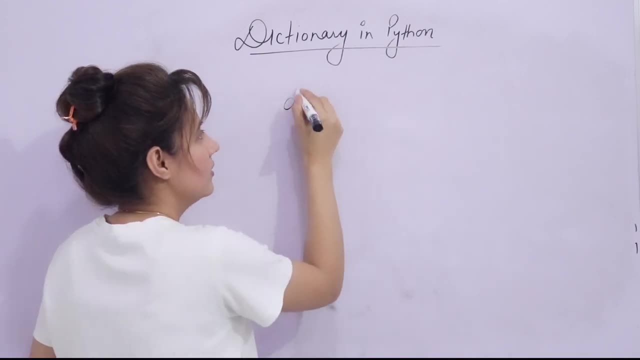 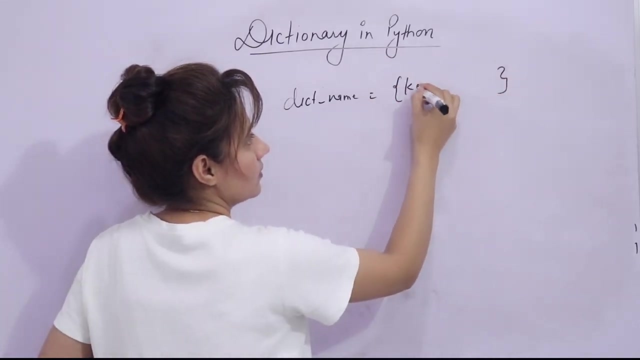 copy, or we can, as it is, do in programming with the help of this data type, right? So what is the syntax, How to store, Just if you want to create a dictionary name of that dictionary, any name equal to, in these braces, curly braces. 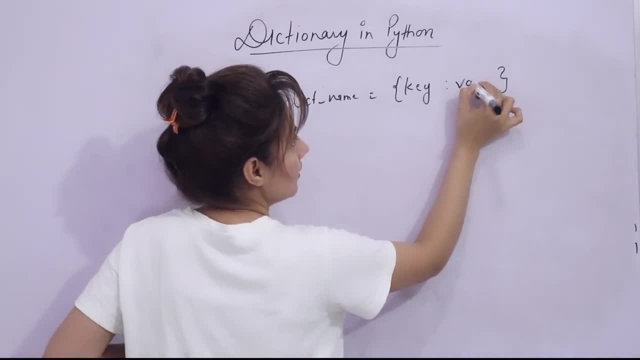 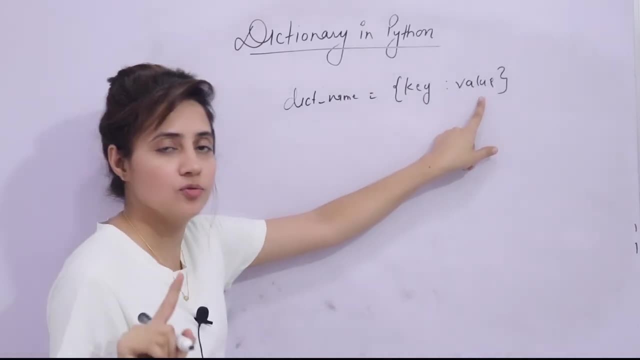 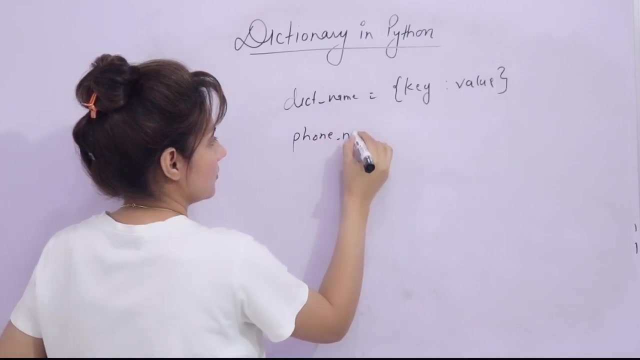 Right Curly braces: key, colon, value. The syntax is very important. First of all key, then colon, then value. This is general syntax. So if I want to store like phone number of my friends, so dictionary name I am taking. 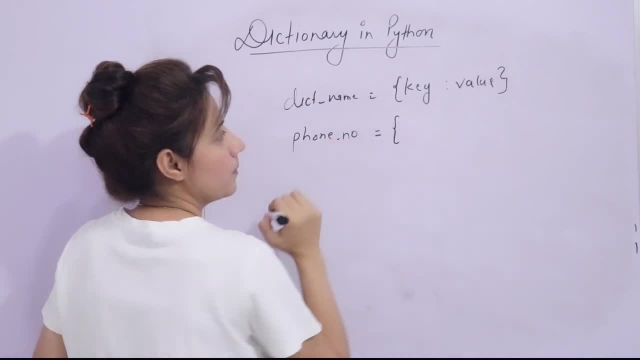 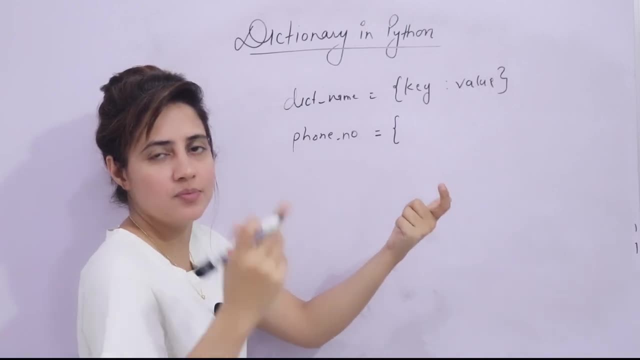 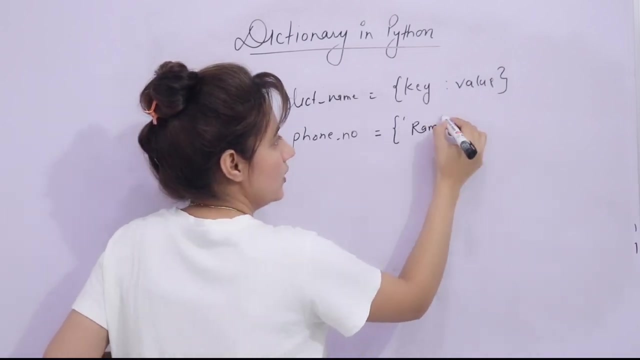 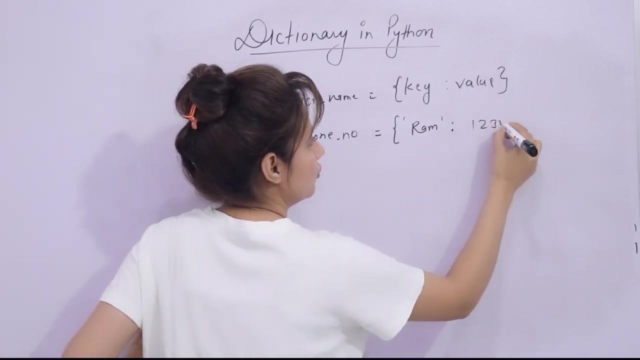 fogon underscore number, and here key Key means suppose obviously phone number. If I want to store, then first I will write name, then phone number. So name is what I am writing, name, Ram. So Ram is what A string. So will in either in double quote or single quote: Ram then colon, then 1,, 2,, 3,, 4, something. 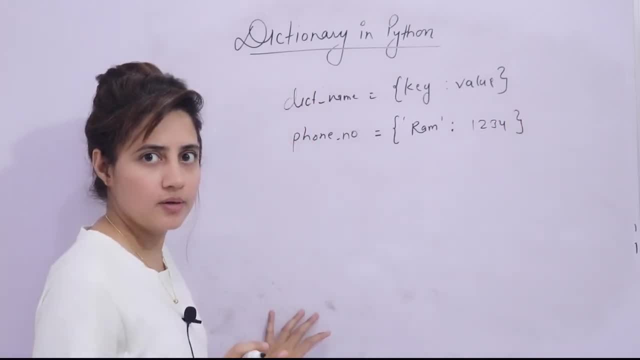 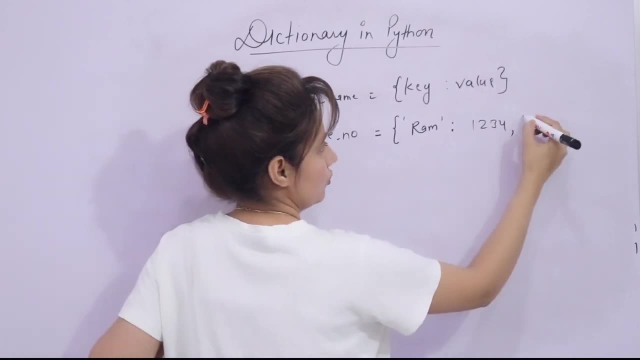 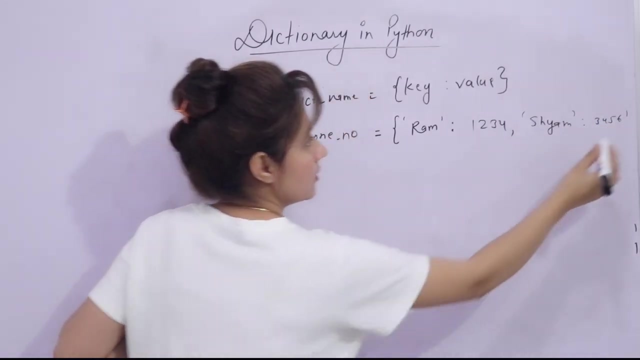 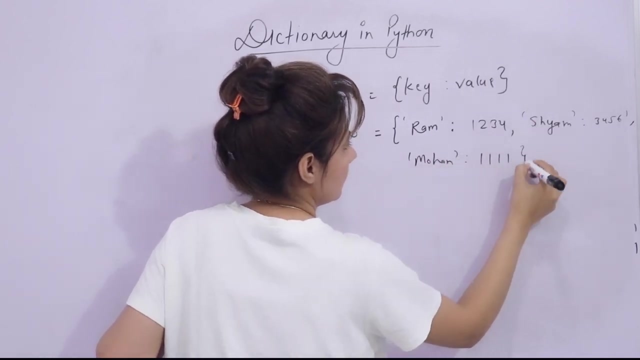 like this phone number. More than one entry is also allowed, just you have to do comma and whatever you want to store Ram and 3,, 4,, 5,, 6 comma, Mohan, 1, 1, 1, 1, any phone number. 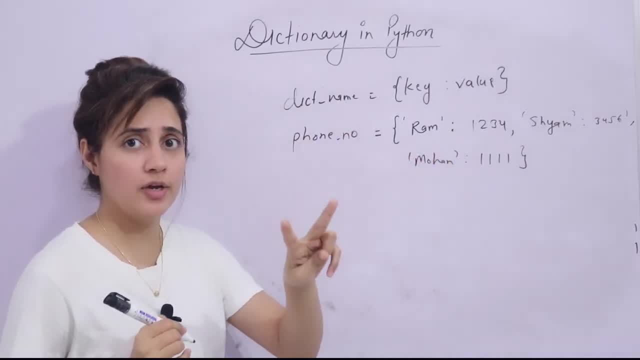 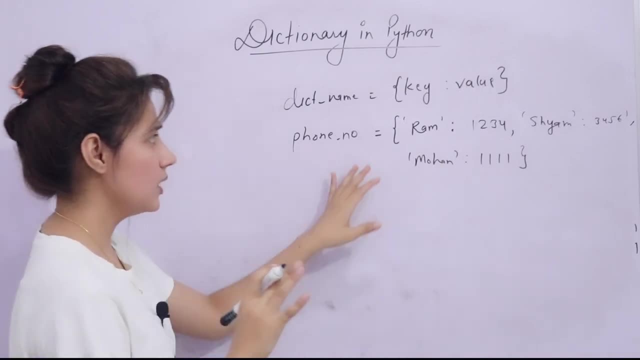 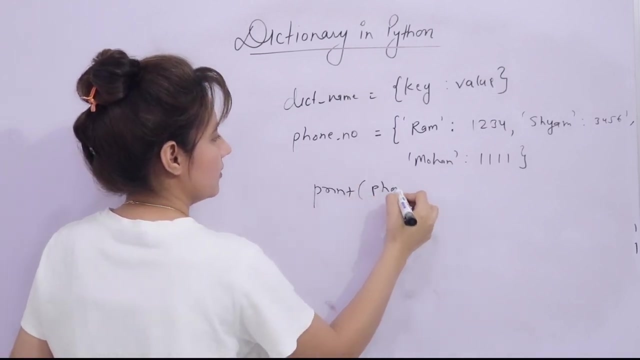 So in this dictionary we are having 3 key and value pair: Ram, this Shyam and for Mohan. Now this is how you can create a dictionary. If you want to access, then simply, we just like this. Okay, Like print and phone number. 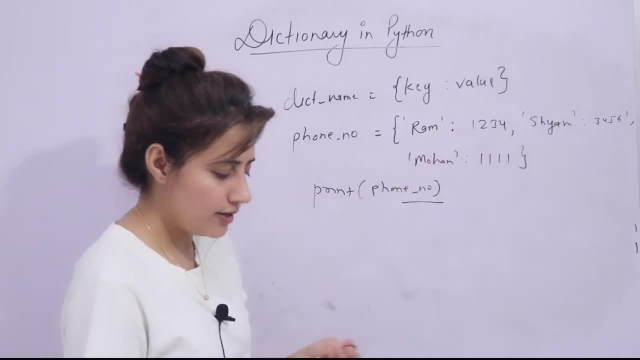 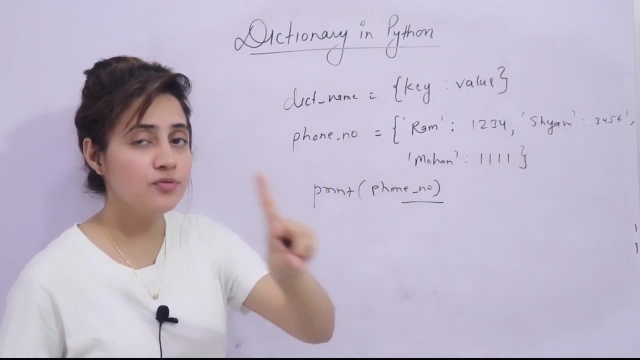 You will get this thing. But there are alternative ways also to create a dictionary. One method is this, The simplest one. We have a dict method. using that also, we can create a dictionary. We can. now we can access individual item also In a list. if you want to access list or tuple, we use index. 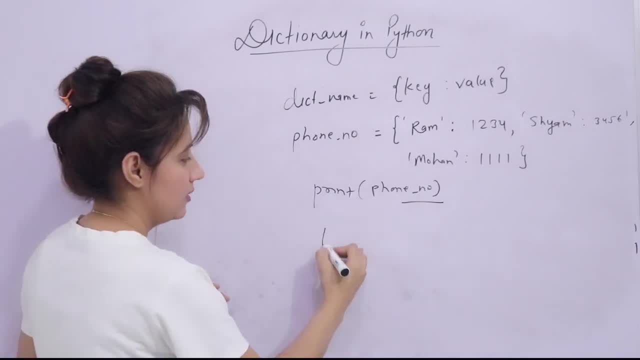 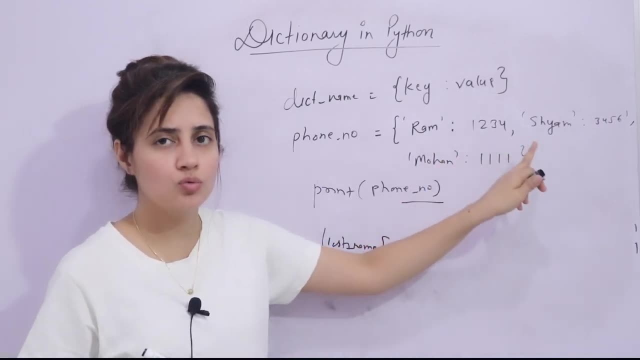 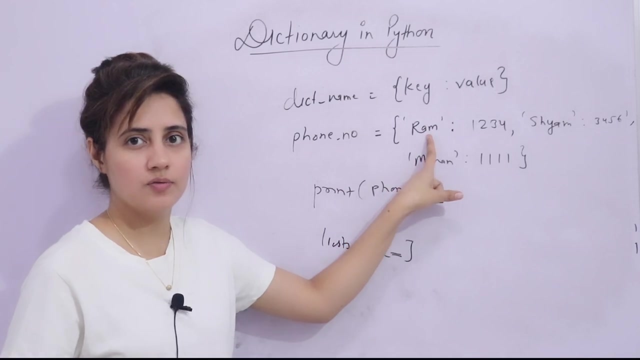 Indexing method we use. Okay, So we have a list. then here we write down list name and then these bracket index 0,, 1,, 2,, 3, 4, corresponding to that index. you will get the value. But here we are having how to access using keys. we are having keys. 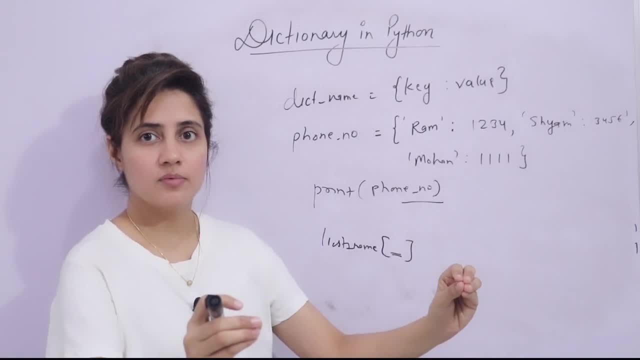 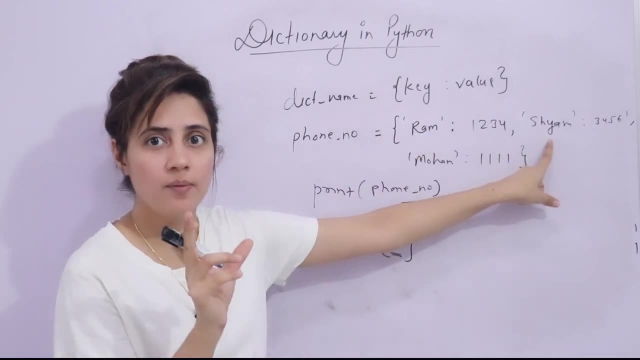 So if suppose I want to find out raw number of Shyam, So what you will look for first of all the name of name of that particular person. So I will look for the name, that is Shyam, the key and corresponding to that I will get. 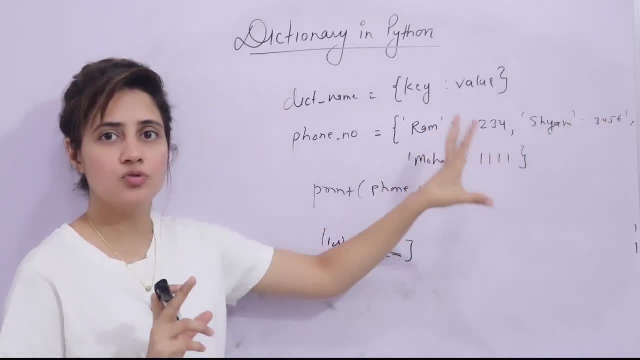 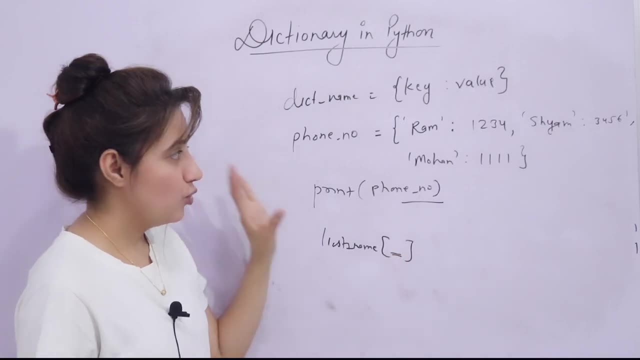 the phone number. So, using keys, we can access individual items or the values from the dictionary, How I will show you Practically. I will show you now everything. Okay, What are the properties of this dictionary that also I will show you when we will do. 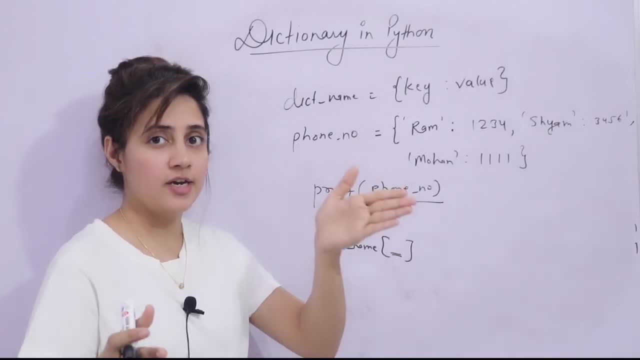 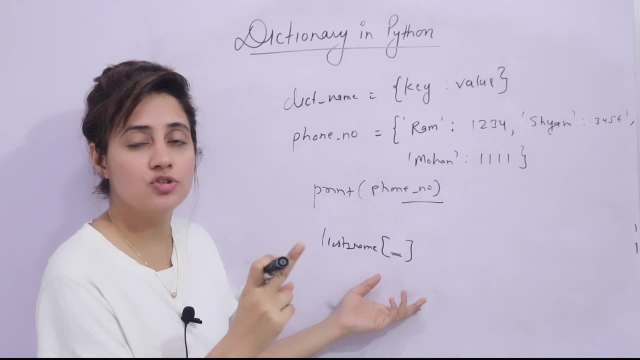 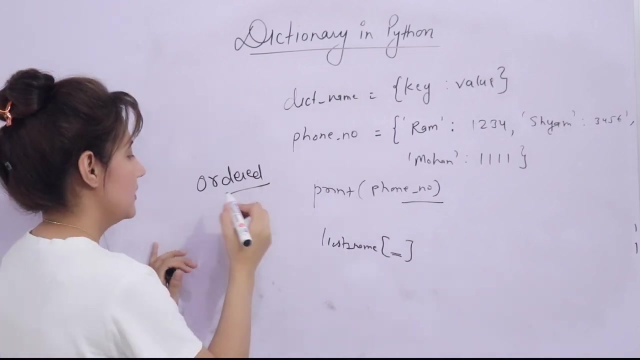 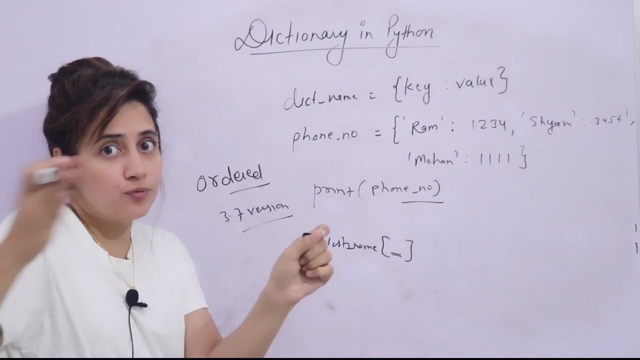 some practical Right. Like for list and set and tuple, we are having properties. So for dictionary also we are having some properties. First one: dictionaries are ordered Right. Yes, Yes, But since 3.7 version dictionaries are ordered In 3.6 version and before that, in earlier version, dictionaries are unordered. 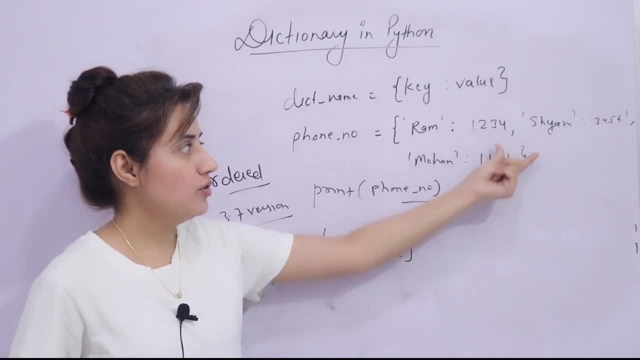 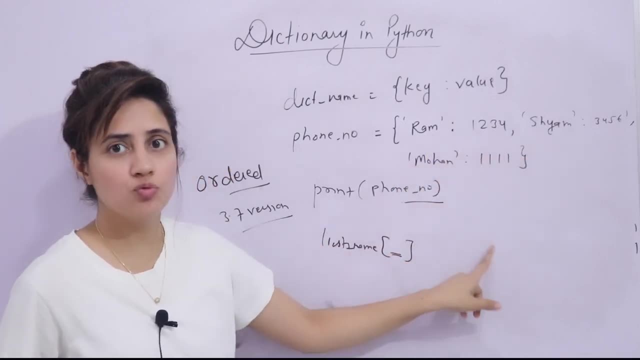 Means. ordered means now you have defined a particular order. now you cannot change that order. If I will print that dictionary, so in the same order these items would be printed: first Ram, this value, then Shyam, then Mohan. It's not like that. I have defined this something like this: 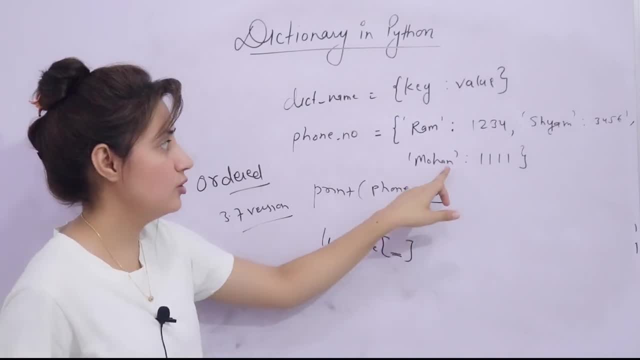 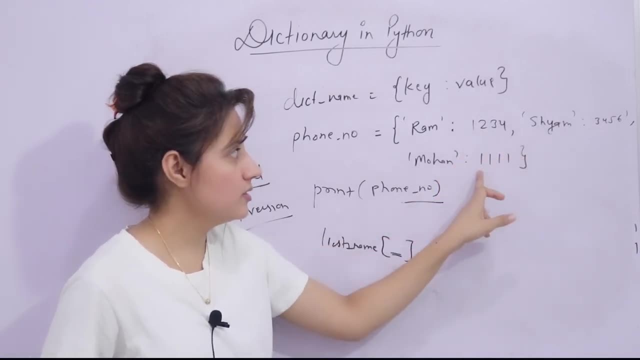 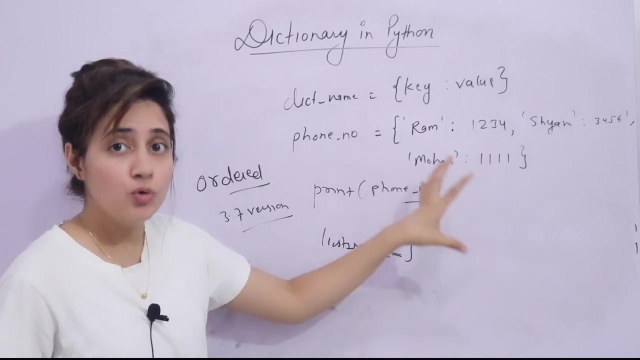 this, something like this: and whenever I print, then first it will give me Mohan, then Shyam, then Ram, or maybe Shyam Mohan Ram. no, whatever order is this, in same order it will print means dictionaries are ordered since python 3.7 version mutable. also, you can change the values if you want to edit the. 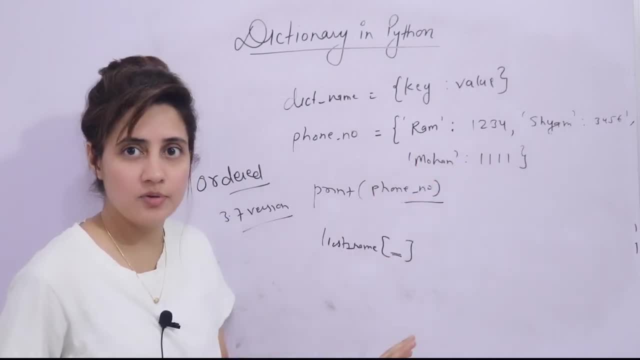 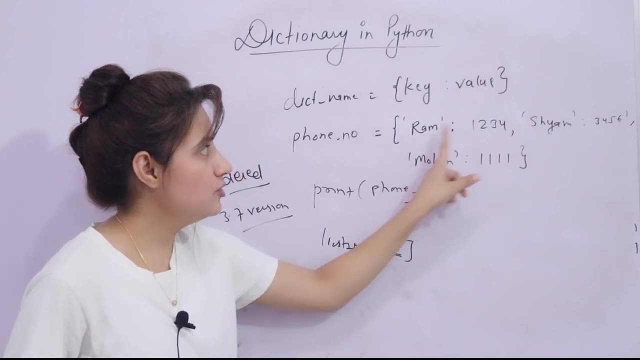 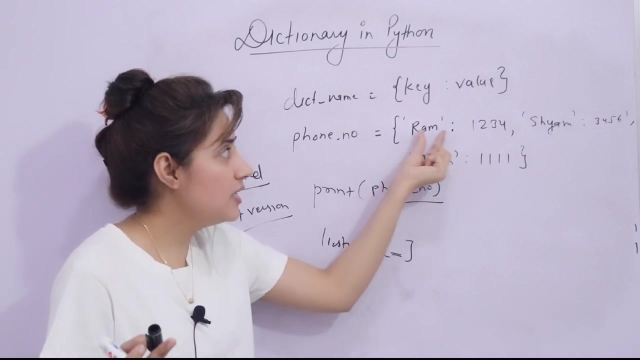 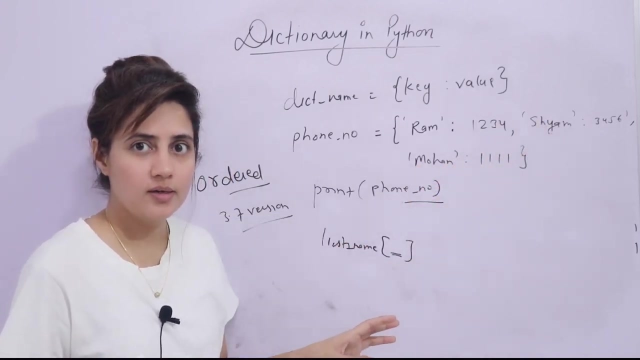 phone number of Ram. you can edit. you can add any item here. you can remove any item. here means dictionaries are mutable, but these keys, these should be immutable. keep this thing in mind. immutable means either a string or a number or tuple. these keys should be immutable, but values are mutable. we can change the values right and no duplicates are allowed. 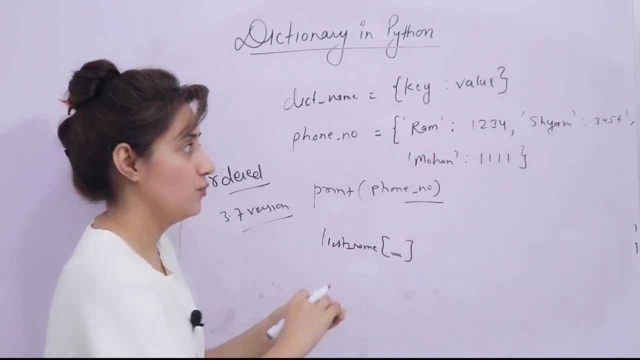 one key can have only one value, like if you want to store. rather than Mohan, I am again writing it as Mohan. I am again writing it as Mohan. I am again writing it as Mohan. I am again writing it: Ram and phone number is this. it's not like that key. this is duplicate key, so this is not allowed. 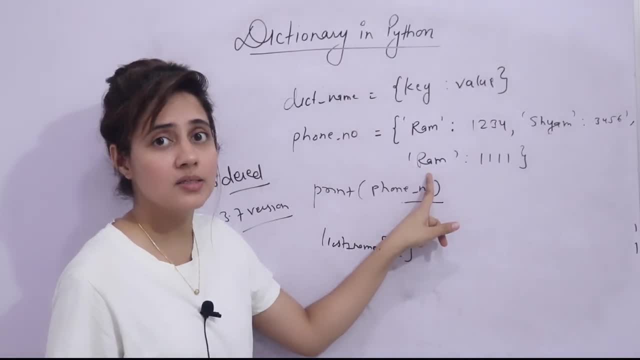 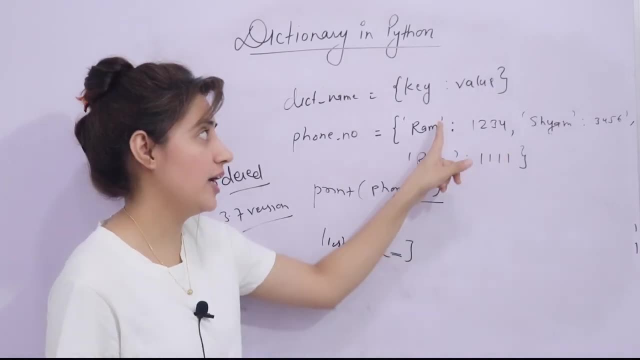 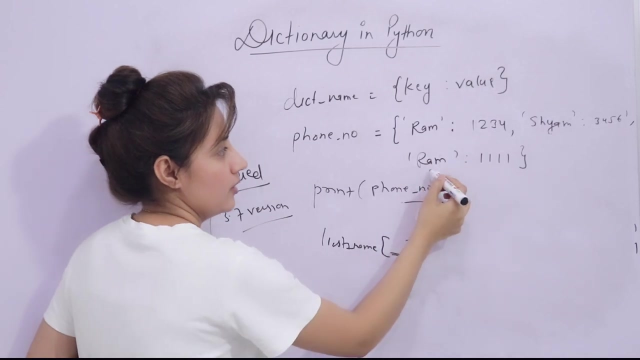 if you will do this thing, no error would be there. but ultimately, whatever value you will assign in the last, that would be considered as final value for that key. so it will only print Ram 1111, Shyam 3456. okay, this value would be discarded the last time. 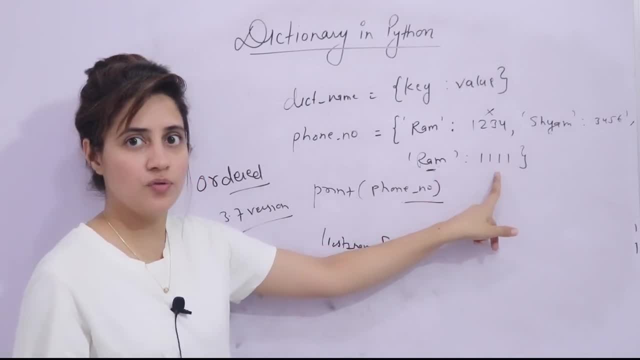 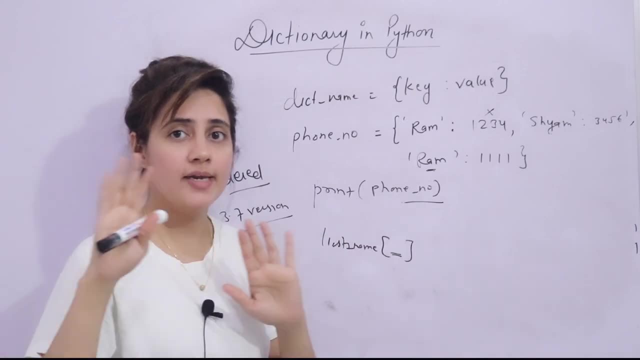 at the last, you have assigned Ram this phone number, so this would be the final phone number, right? so these are some properties. okay, now, basic idea. you will get the syntax and all. now let's do some practical of these things and, just you know, find out what different, different built-in. 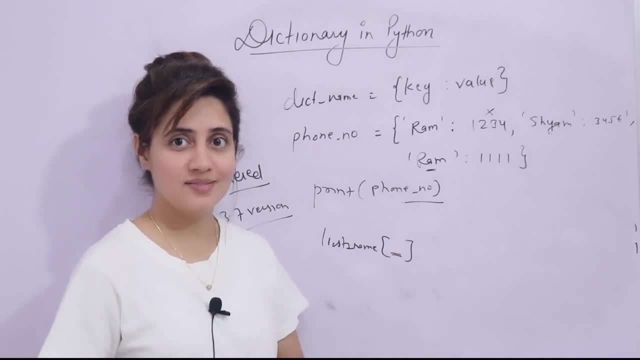 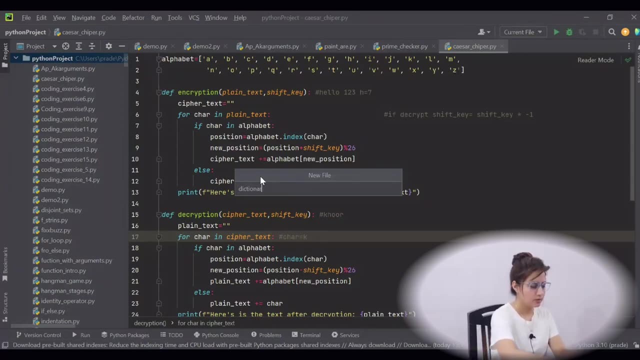 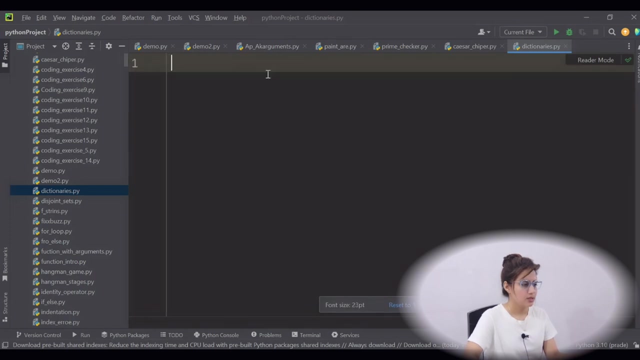 function we can use here. many built-in functions are there, right? okay, so let's create a new file here and dictionaries dot py- this name I am taking. let's create a dictionary- any value or any information you can store. I am just taking an example of storing phone number. 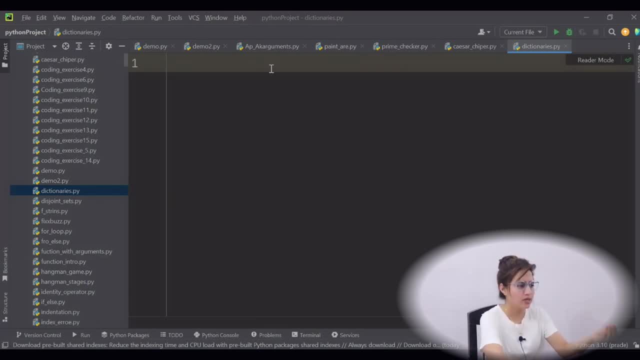 any value which is in the form of key and value like student name or number or anything, or like information of employees: name, then age, then phone number, something like this, anything you can store. so So I am taking phone number. simplest method is: name of the dictionary: this curly braces. 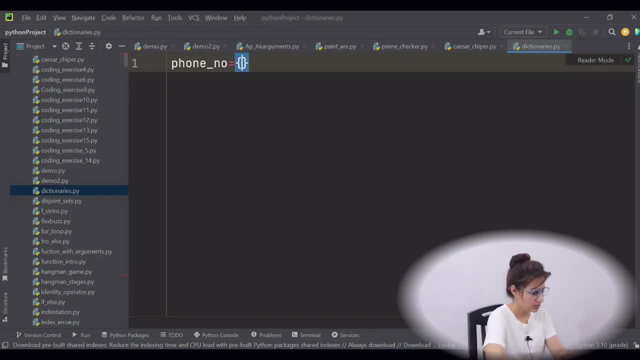 and then first suppose I am writing name. this is the string. so definitely it would be in curly bracket. sorry quotes, double quote or single quote, then colon and then value like 1,, 2,, 3,, 4,. this is the phone number. ok. 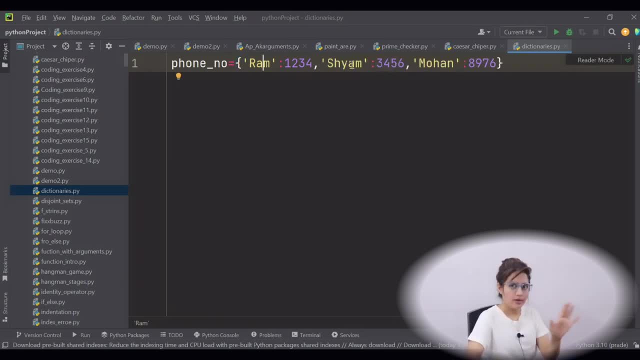 So three items I am having. so yeah, that is, it is ok. it will not give any error. but according to the you can say convention is there in Python whenever you will write dictionaries, If suppose we are writing something like this, if I am having definition of something like: 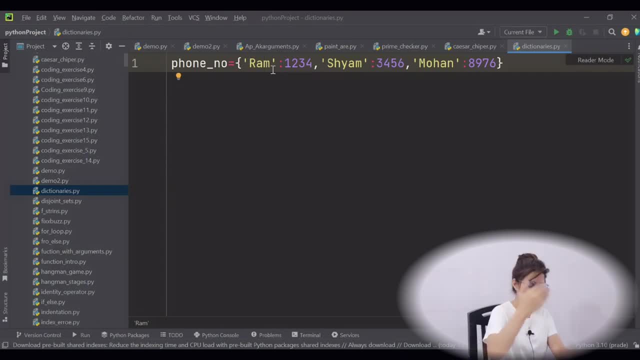 first definition of code or definition of algorithm. so here I write algorithm and then here I write definition in one or two line, then comma, definition of program, then definition of code. So it would be very, you know, It would be not so readable if you write down just in single line like first algorithm. 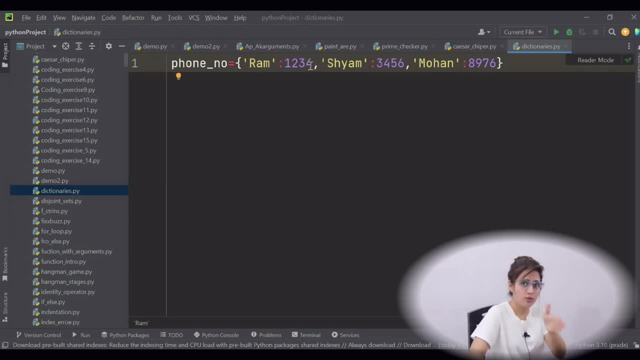 definition of that, then comma from there only start another item. no. So what is the convention for more? to look at a program more readable: Generally in Python we write simply: first curly braces would be start in first line, then with some indent: first item, comma. then in next line second item, then comma. 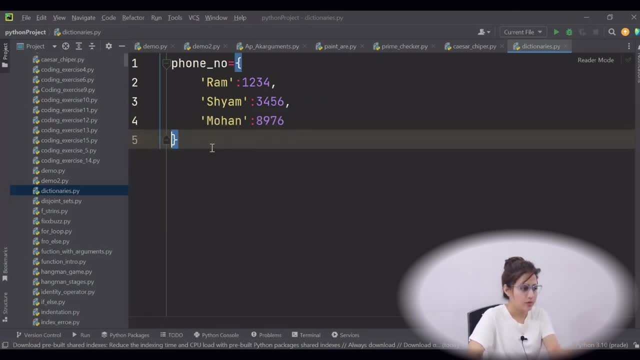 2,, 3,, 4.. in third line, third item, Then, at last, with no indentation, we will close the dictionary. So this is the convention, Although if you write down everything in one line, that will not give any error. but this is more reliable, right? And if you want to add another item, 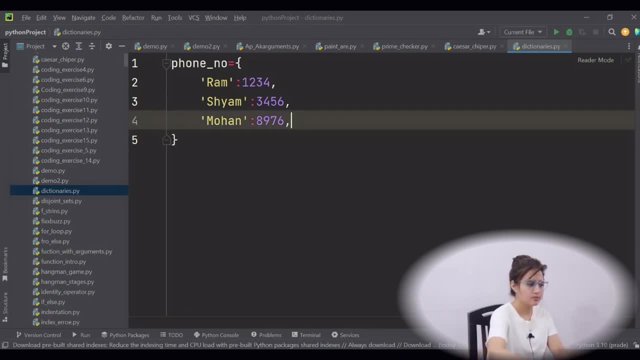 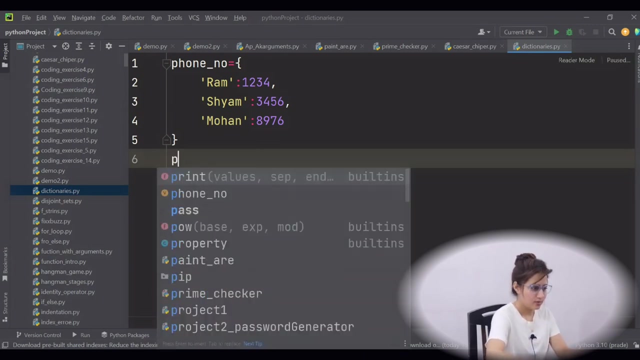 just comma enter. you can add another item right. Or if you like to put comma in the end, that is also fine. It will not give any error. okay, So let us run this. okay, Because we have not printed anything, so it will not print anything. Let us print this dictionary. 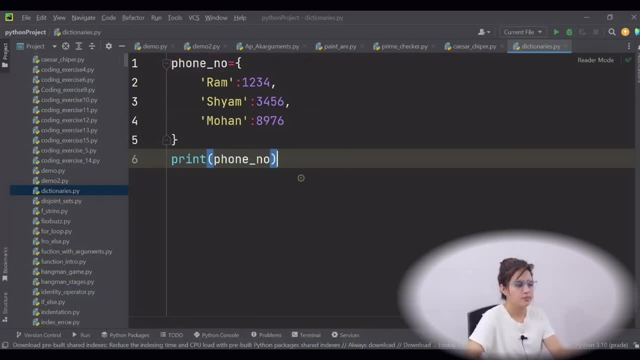 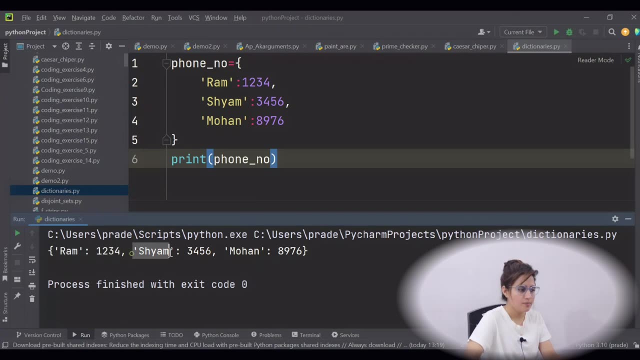 print and just name of dictionary phone number. that is it. So let us run this and see. It will print like this: This Ram Shyam and Mohan key and value pair everything. If you want to access Phone number of a particular you know person, you have to provide the key. If any specific. 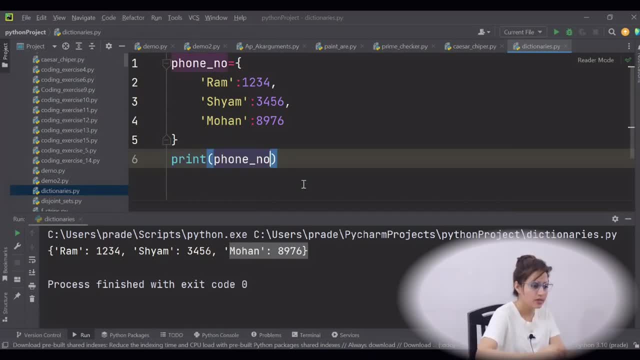 item you want to index. specific value you want to access, then name of the dictionary. in these subscript brackets no index, because in list and tuple we use index. Here we write down key, So just write down the name of that person. Suppose I want to access phone number. 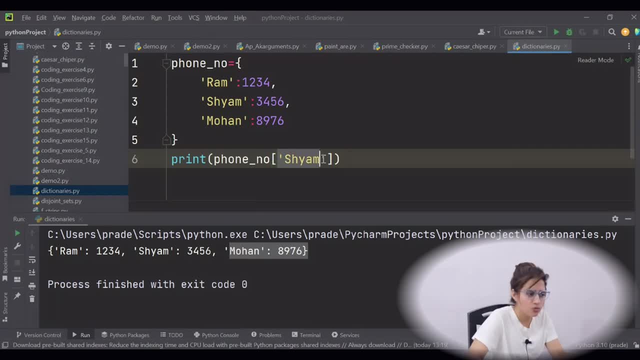 of Shyam. See, Shyam is string, So as it is, you have to write down the key: Shyam is a string, so in quotes. And second thing: case sensitive. This is case sensitive, so you have to be very careful If you have. 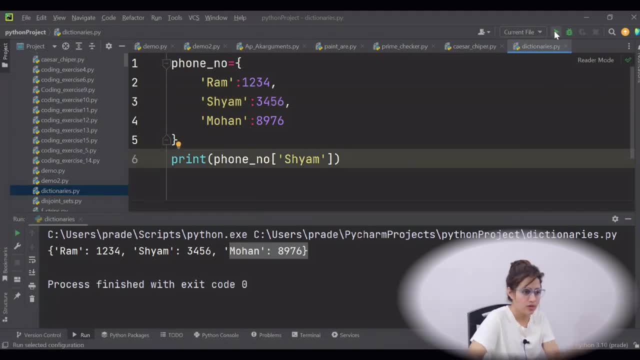 written this: S capital. this should be capital, right. So let us run this and I will show you. See, phone number of Shyam is 3456, right. If you write down something like this small s, Let us run this, It will give you a error, See. 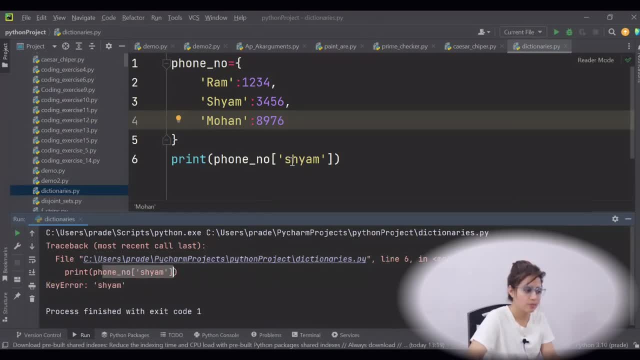 Key error: Shyam. In line number 6.. In line number 6 I am having a key error Shyam. So this is the common mistake generally. you know many students do Just a typo error. So you have to keep in mind this thing: The key name it should be same and if it is a string it. 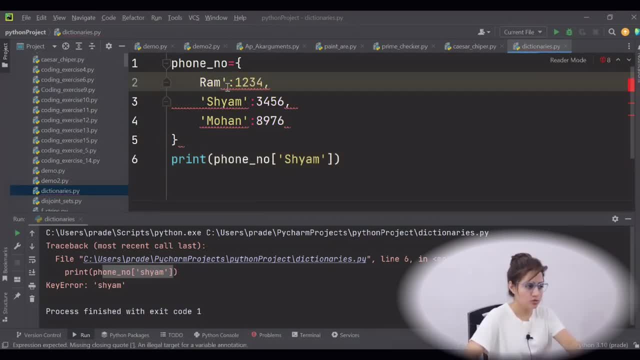 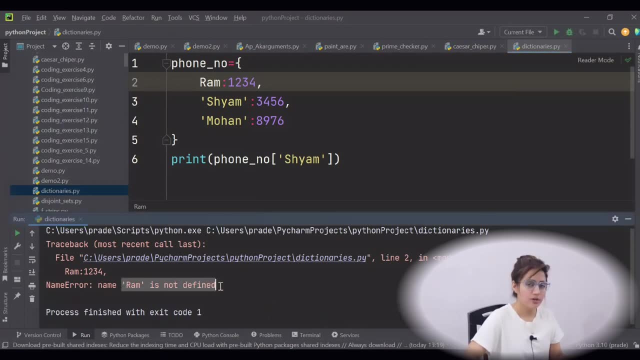 should be in quotes. If you will not put here quotes, it will give error. Let us run this. See, name Ram is not defined. Okay, So if it is a string, so you have to put it in single quote or double quote, right? If it is integer, that is fine. Next thing, next: property of 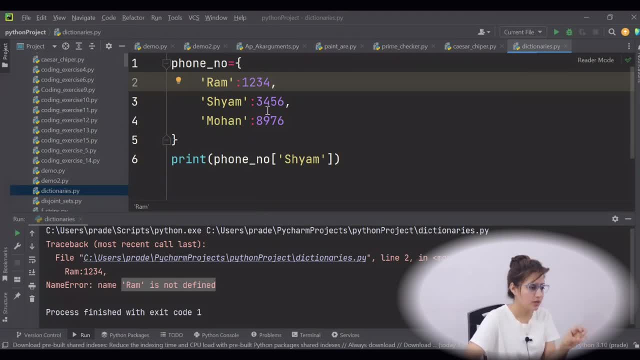 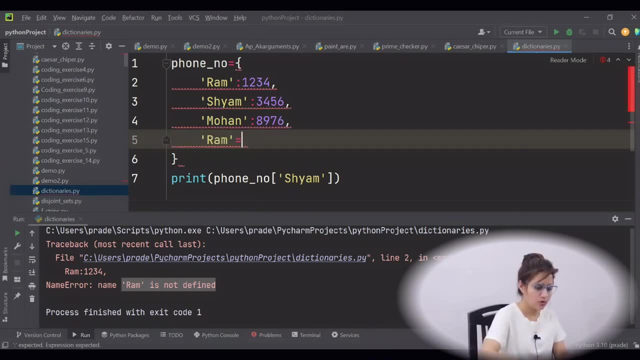 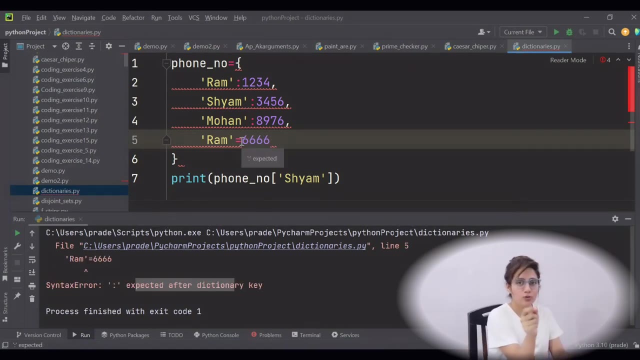 this is what. This is how you can access particular item. Next, I have told you duplicates are not allowed. So again, if I assign Ram equal to and And 6, and yeah, there is, and see, this is also- you cannot write down here Ram equal to 6666. 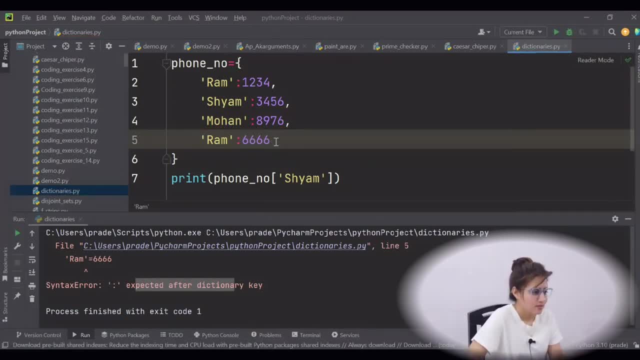 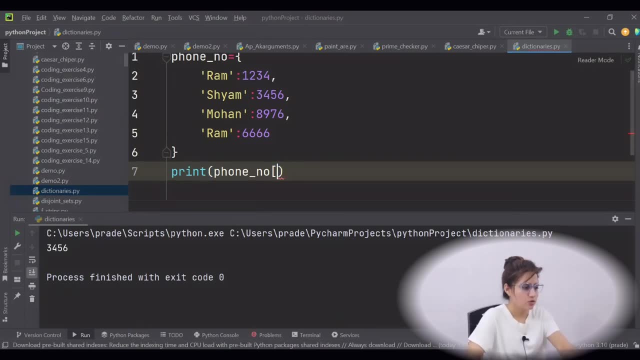 It should be colon. I have told you the syntax, So this is also one of the common mistake. Okay, I am just getting this one. So let us print dictionary the all the values. Let us run this: all the items: See Ram. the phone number of Ram is now 6666.. It is not 1234.. 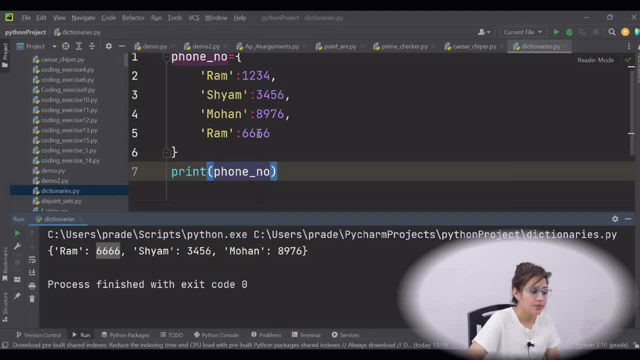 I have told you. If you do so, if duplicate keys are not allowed, If you do so, if duplicate keys are there, then whatever value you will assign in the last, that would be the final value of that key. So 6666.. Right, Only one time it will take. 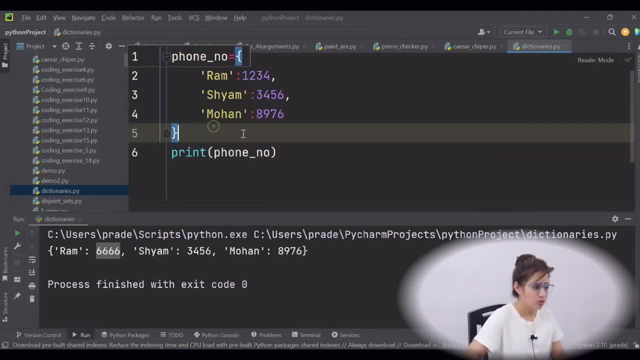 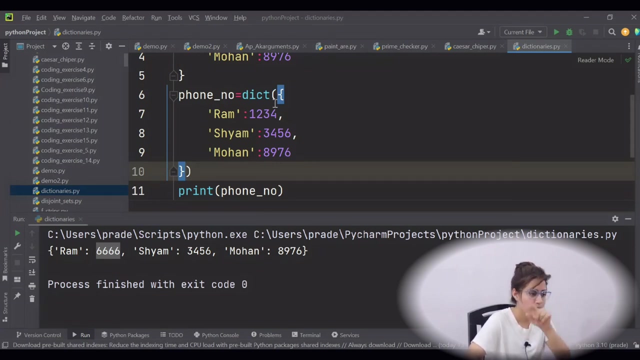 Ram. Okay, Next property is what? Now we have another method also to create this dictionary, Just phone number equal to. we have a dict, function, Dict, And here you can pass this value, these items. So I am just copy pasting these Dict that brackets Right Round brackets: 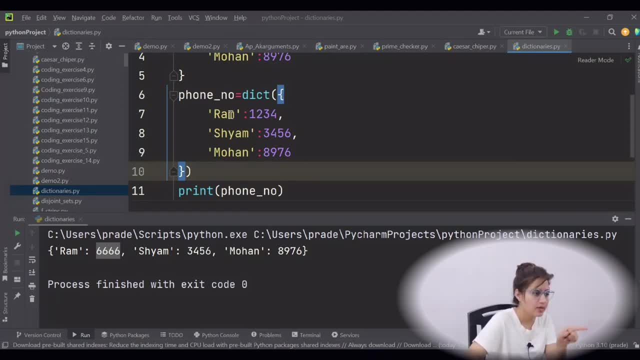 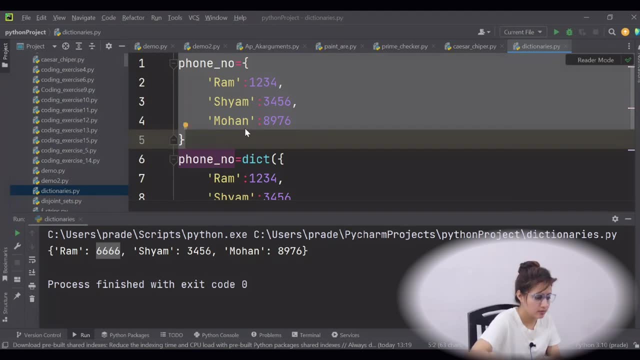 And then, as it is, you can pass whatever you want to write in dictionary, Curly bracket, then key and value pair. Key and value pair. Key and value pair. Right, So if I comment out the previous one, and this is our final one using dict, So it will give you same like. 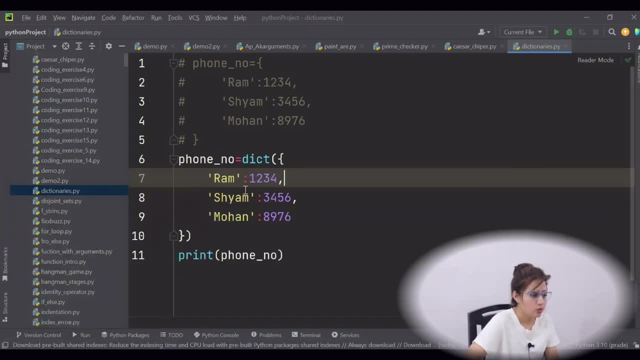 this. So this is the second method. Otherwise, you can also pass each item as a pair. This is the complete item Key and value: complete one. This is one item. this is second item. this is third item. So this one item you can pass as a pair. Something like this Now in: 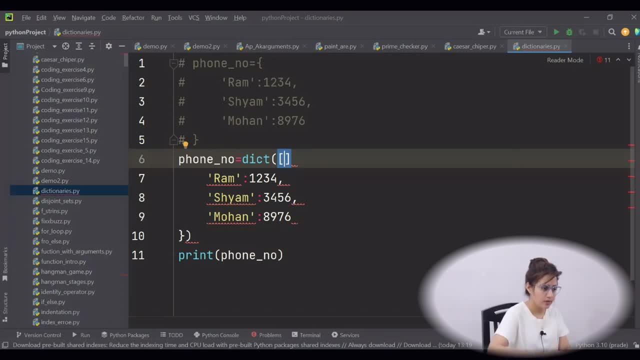 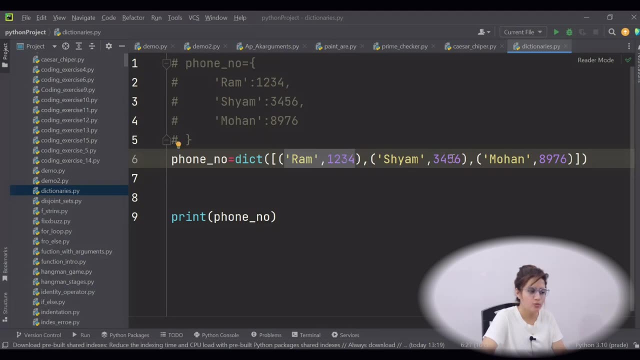 this case, rather than curly braces we use square bracket Right And like this dict: then each item you can pass as a pair: Ram comma, the value. sham comma, column Right: This one is a number. Mohan comma, phone number, in round bracket and this value: Sorry, this. 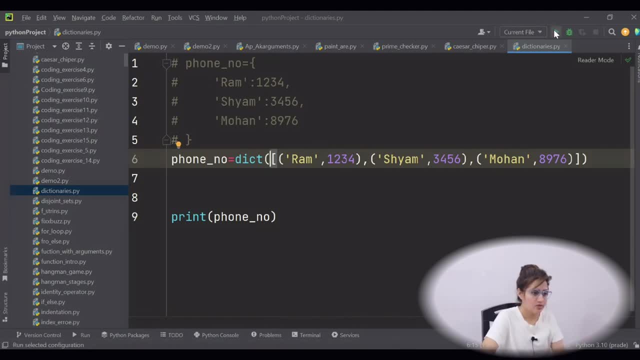 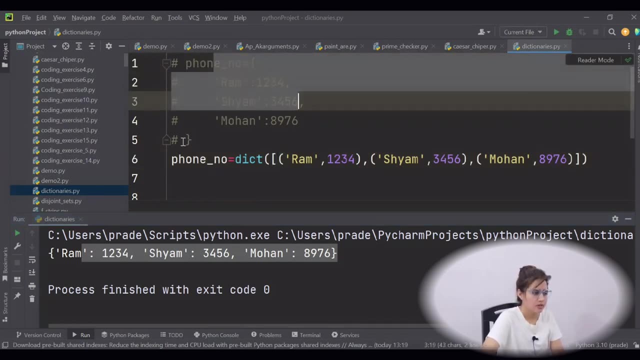 bracket, square, bracket Right. Okay, let us run this, and this will also show you the same. So these are some methods to create, but the simplest one is this one, So we will use that only. Let us just comment this out. We will remove the comment of this Now. next, 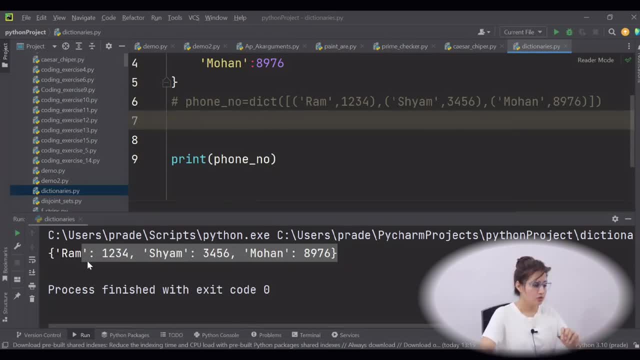 is Okay, I have told you, these are ordered. So not only this, but these are ordered. For example, we will also create some objects, So some objects. So, for example, we will create some objects, So let us just remove some objects. So let us remove some objects, So let us remove. 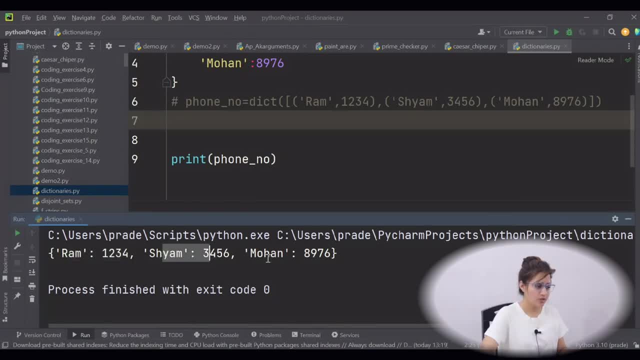 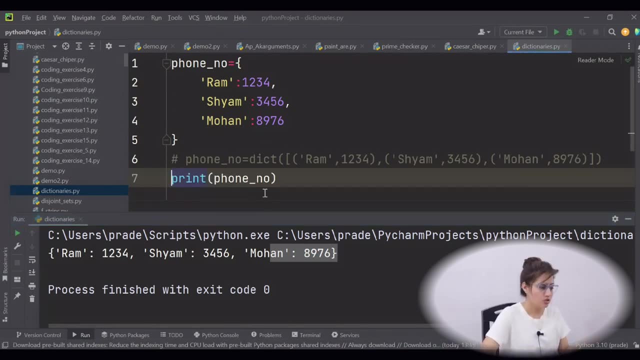 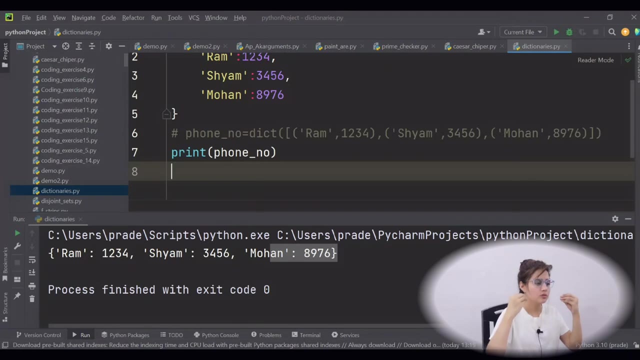 see, in the same order it is printing, The first item is Ram, then Shyam, then Mohan. So in the same order it is printing, Next is mutable. Okay, So the values are changeable. Now if I want to change the value of the phone number of, suppose, Mohan, I can change How. 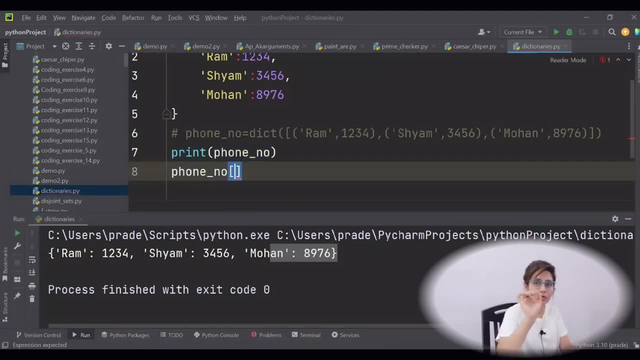 Just name of the dictionary in the square bracket What key For what you want to change the value? Just pass that key as it is Mohan. same name, then sorry, then equal to, and whatever the phone number you want to assign: 9999.. Okay, Now I will print the dictionary again. 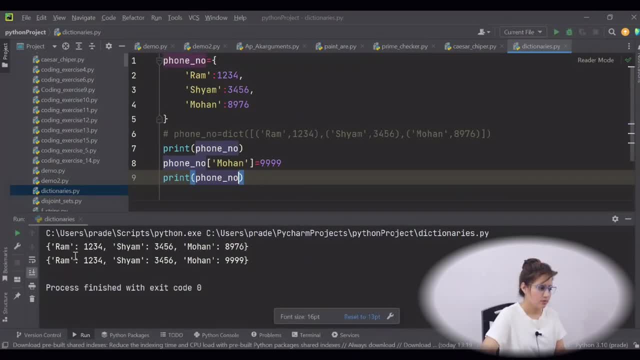 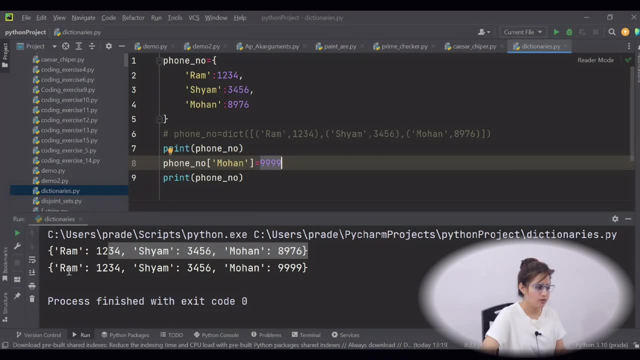 Okay, So let us run this again and see: At first the same, whatever you have assigned. then we have updated phone number of phone Mohan- and then see the phone number Mohan is 9999.. So this is how you can update any item. 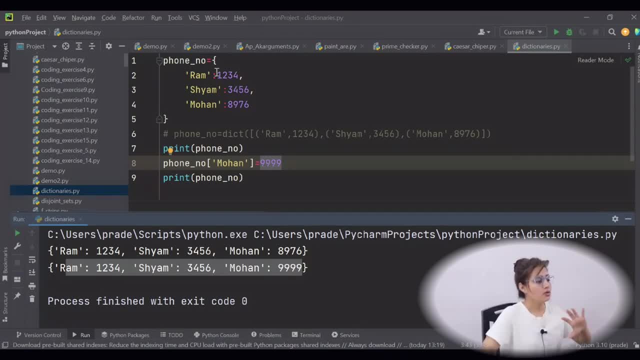 Okay, Next is okay. Now the values are. these values can be of any data type. See, I am saying values can be of any data type. any int, float list, tuple, dictionary set. anything But these keys should be immutable. 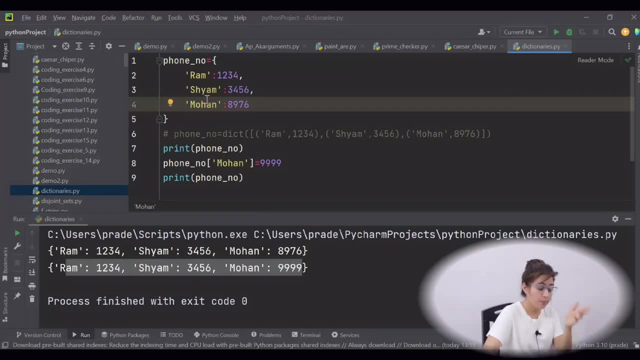 immutable means either number or list- sorry, numbers, tuples or strings. these are immutable datatypes, right? So here, a dictionary can also contain list, as well as a dictionary itself, dictionary inside a dictionary, nested dictionary. So let me just show you Now, rather than here, Mohan, one thing I want to add a list. Mohan is having two phone number, so I 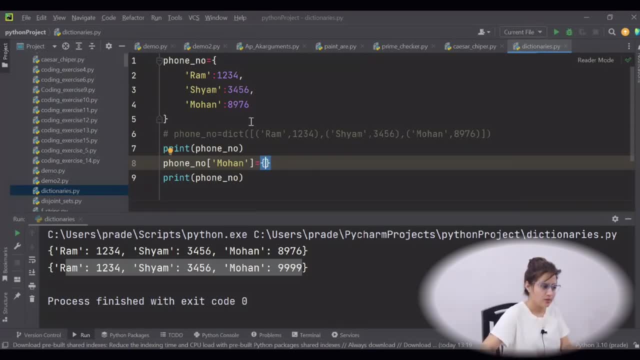 am adding a list of phone number, whatever Mohan is having, rather than this one, or I am not changing. I am adding one more item, sorry, one more name, and that is Madhav, and for Madhav I am adding two phone number: 1111 comma 2222, or suppose I am adding two phone. 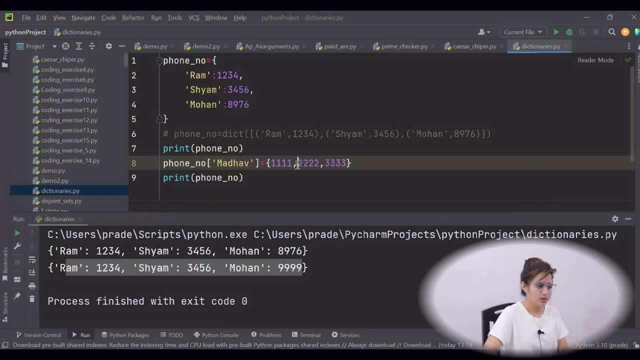 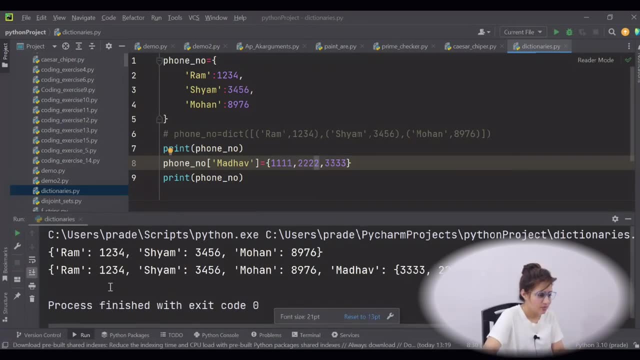 number 1111, comma 2222, or suppose three phone number 3333.. So this is a list of phone number. that is also fine, you can add. let us run this: see before updation. this is a dictionary and after that we have one more item, Madhav, and this is the thing. So list is also allowed. 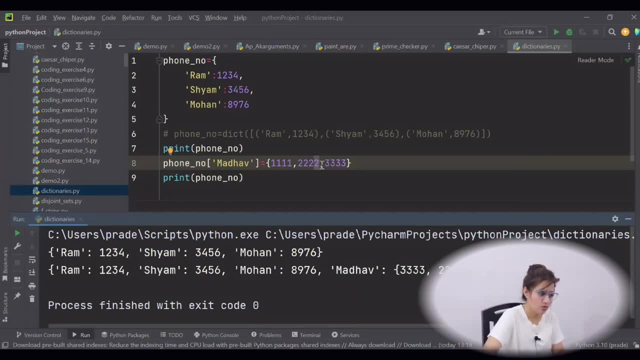 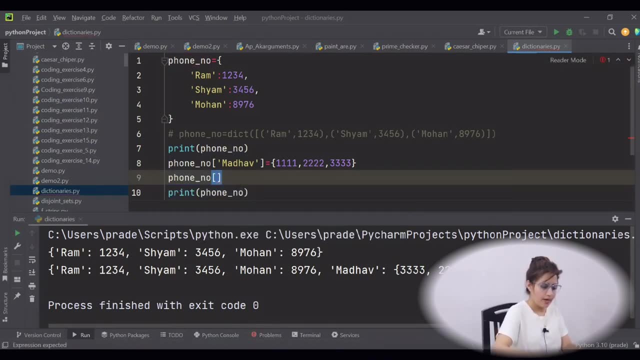 it is not like that you can only write down here maybe integer or string and all. no, even dictionary is also allowed. one more item: I want to add Phone number and suppose I want to modify Shyam. Shyam is having two phone number and 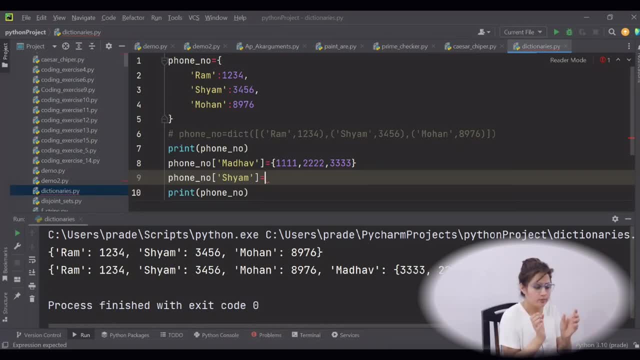 I want to add these two phone number in the form of key and value pair: Shyam home and Shyam office. right, this thing. So that is a dictionary: key and value pair. this I want to add, and then let us print phone number. let us run this. see, first one is with the: 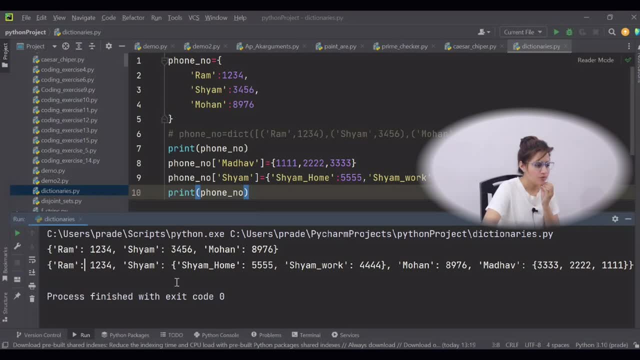 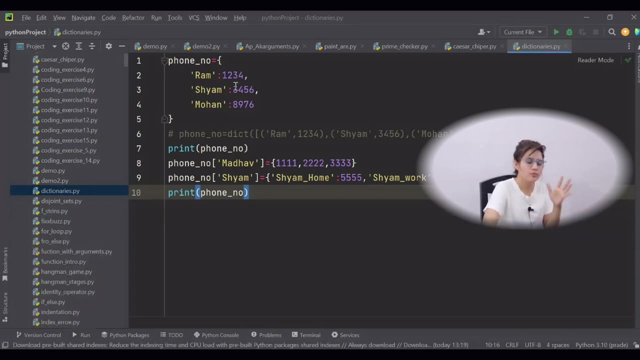 without modification. then we have added Ram for Shyam, we have updated see Shyam, and then this is having a again dictionary: Shyam home, Shyam work, then Mohan, then Madhav, like this. So the values can be of any data type right Now. if you want to access, suppose, if you want. 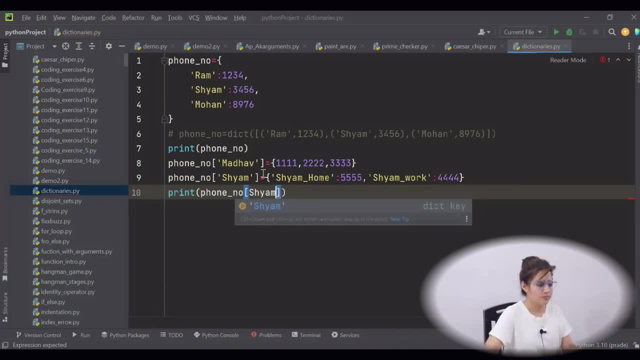 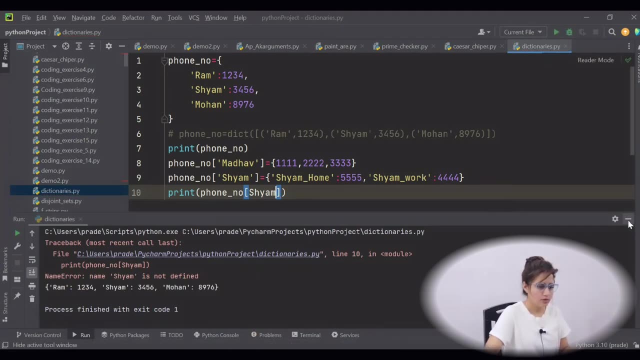 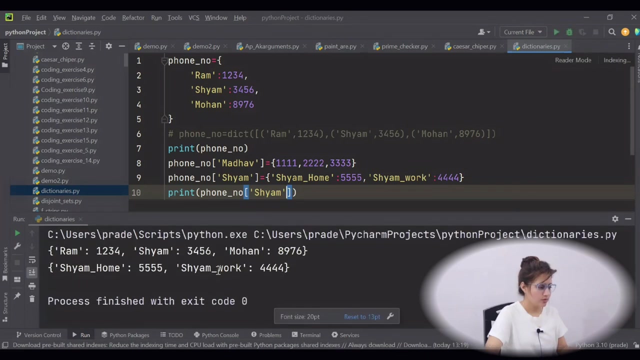 to access this phone number of Shyam. see what it will print. Okay, Shyam is not defined. this is string, so you have to put in quotes. See first of all, we are printing this phone number, the complete dictionary. so this is the first print. 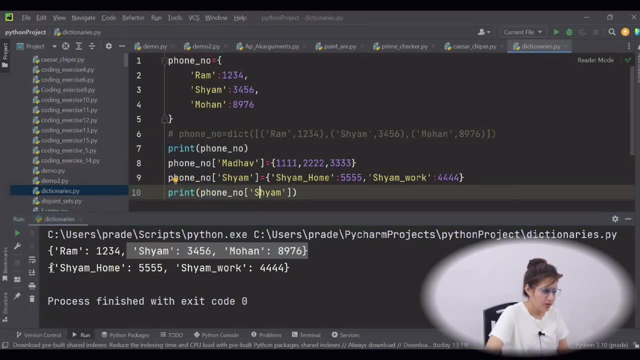 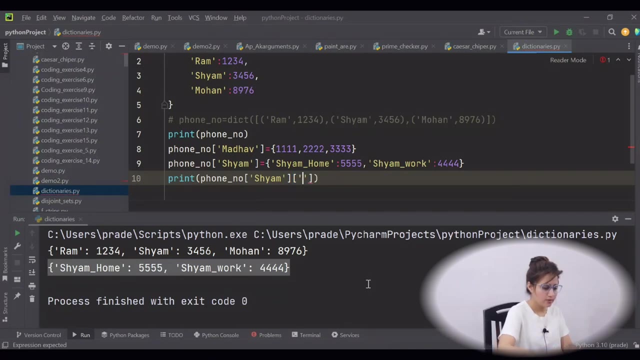 statement and then for Shyam I am printing. so this is the second print statement. So Shyam is having two phone number in the form of dictionary, this and this. So if Shyam work, I want to access then what you will write Shyam here. then again, here I will write Shyam. 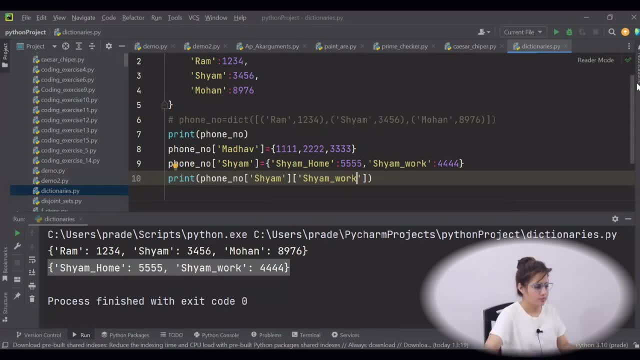 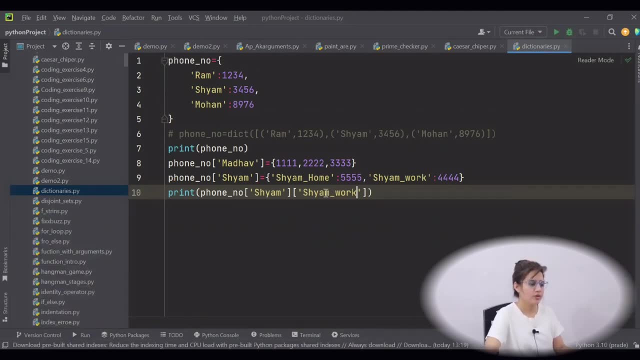 underscore work. let us run this and it should print: 4444. see, So this is how you can access. okay, using get method also, we can access these things. So let us print. we have how to use that method. phone number. Okay, Dot get, and here same for which key you want to access the key name, it is Ram. Let us run. 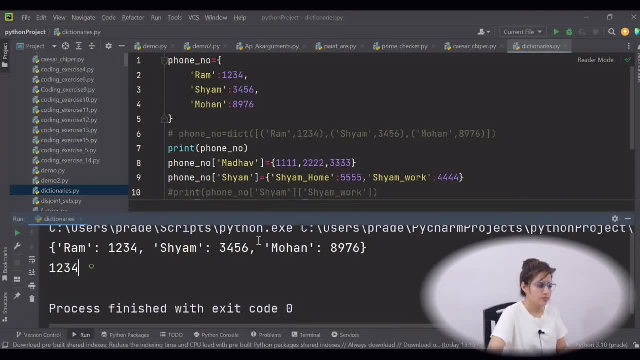 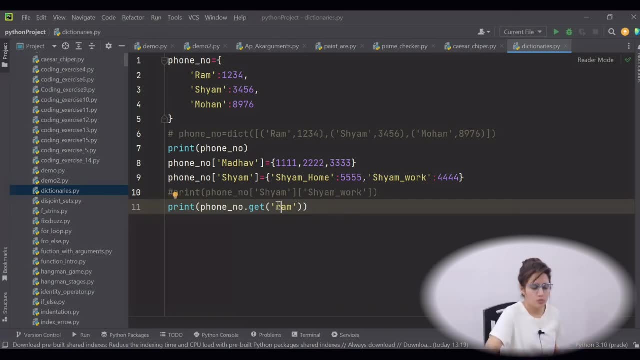 this: see 1,, 2,, 3, 4- right. But one problem with get method is what if I write down here: suppose small ram, So if you do not use get method, then it will give error, key value error. this is not here capital Ram, is there right? but this will not give any error, it will just. 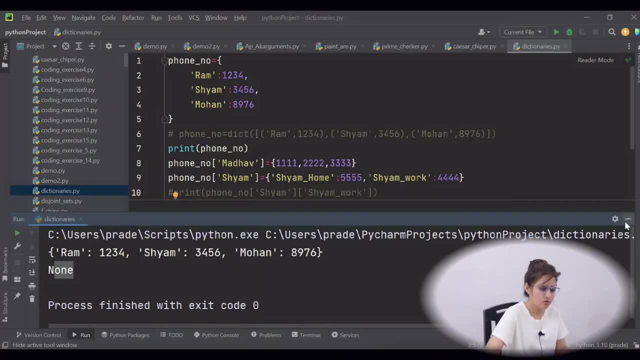 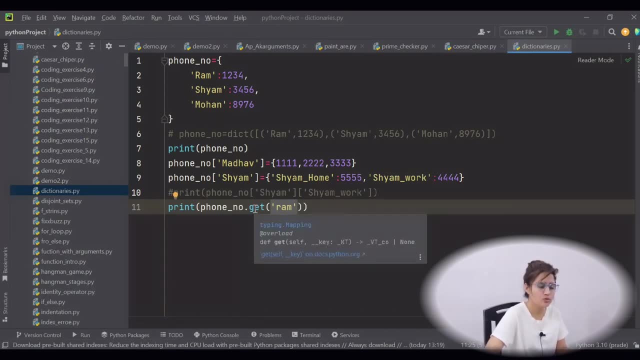 show you none. So if you want, like some error should be printed, if I, if I write down here a wrong key, then definitely we will not use this get method, previous method, we will use. okay. Okay, I have one assignment or a question for you. If this is a dictionary data, which is 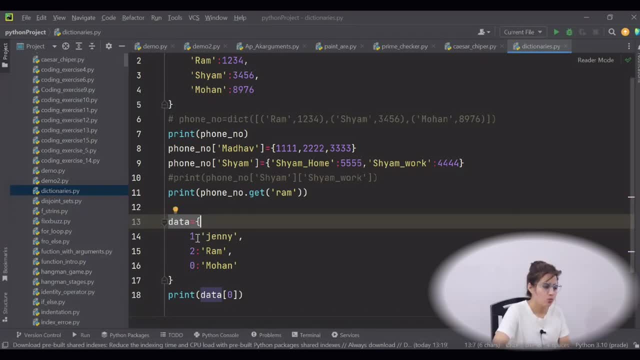 the key of my data. this one Data I am having: 1 is the key and value is jenny. then 2 Ram 0, Mohan, and I will print data and here in subscript I am passing only 0.. What would be the output of this thing? Pause the video and think So what it will print. See 0 here. 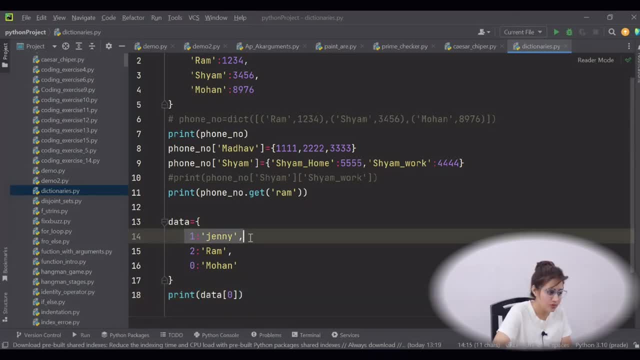 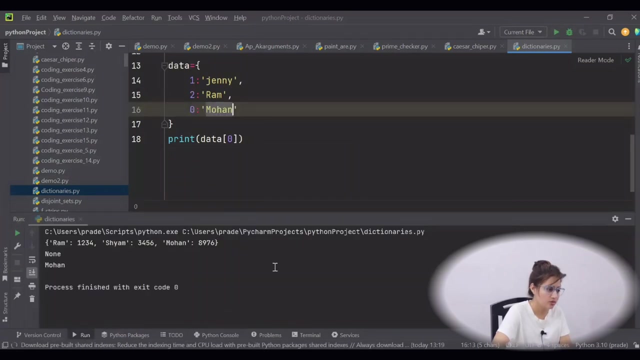 is not index. So do not think, at zeroth index we have 1 jenny, It will print this one. So this thing No 0 here is key because we are accessing dictionaries. So key, key is this thing: this is 0.. So it will print: Mohan, value this, Mohan. Let us run this, See it. 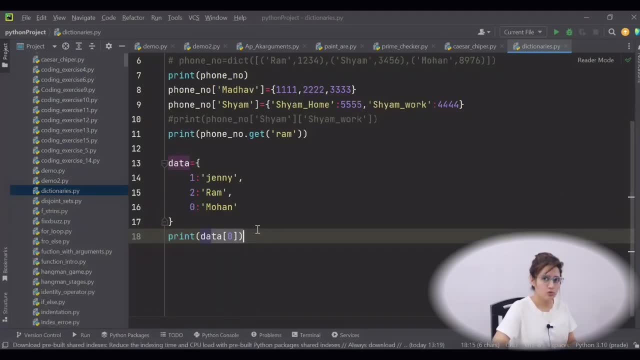 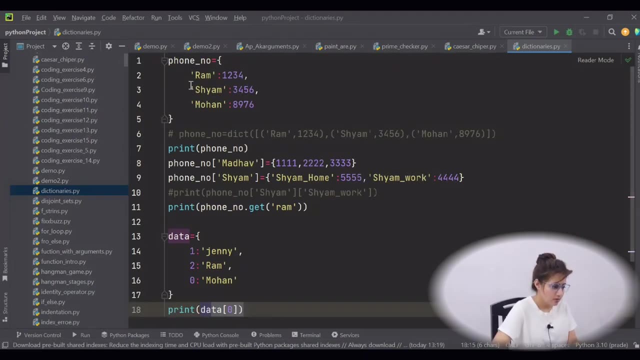 is printing Mohan. Okay, I hope you got this thing also. You also will not. you know mistake. you will not do this silly mistake. So here the second. second is what? Rather than this string here in keys, I am using integer, So that is also allowed. It is not like that. 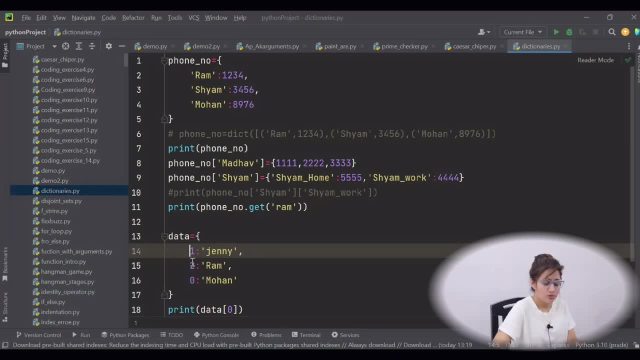 only string I can use, Okay, String, integer- sorry string- or numbers or tuples we can use, because these are immutable List. we cannot use List as key. we cannot use because list are mutable. Now, if you want to delete, if you want to delete any item from this dictionary, 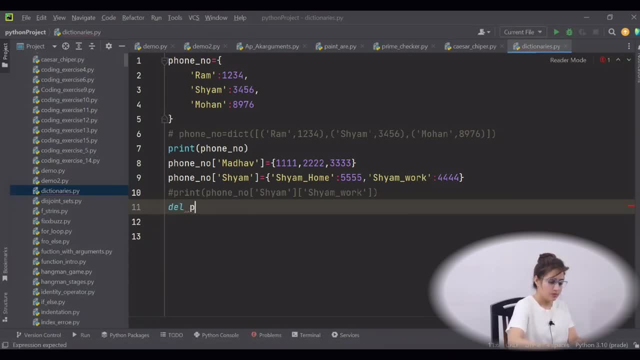 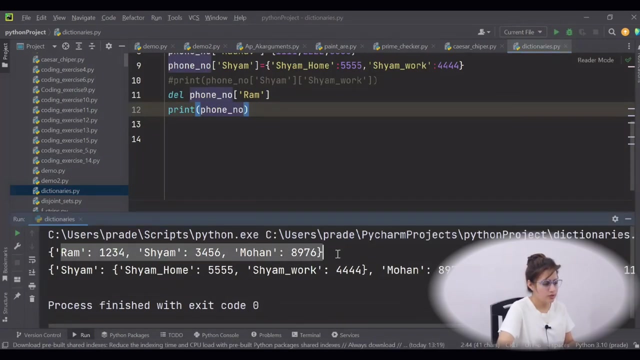 we have a method, del, Del, just name of the dictionary and name of that key, what you want to delete, like RAM, and then if you print phone number, then see what it will print First is this one without updation. then we have deleted RAM. then see there is no RAM. 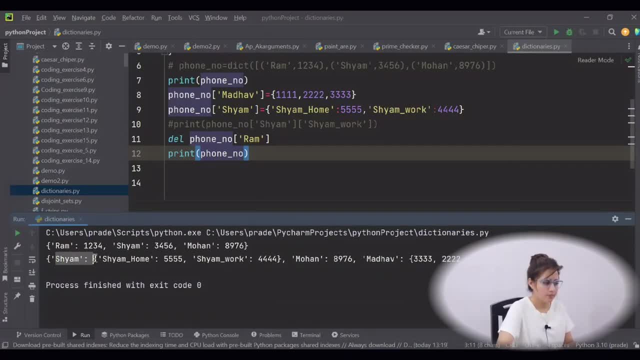 At first. I am having Shan. This print will because we have deleted RAM here, So that key and value, that would be deleted. So using del, we can delete. Using pop also we can delete. How we can? you can delete that thing. See, you have to use name of the dictionary phone. 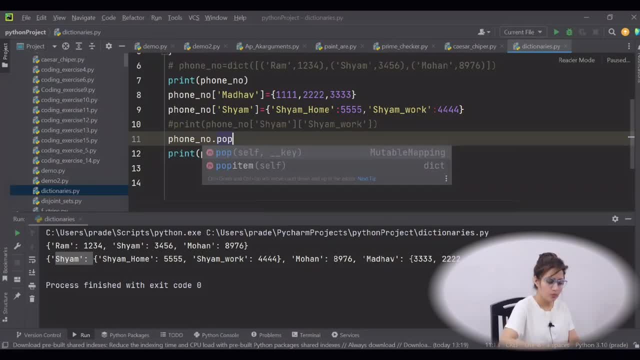 number dot, pop function. we have pop and here save, Okay, So that is all. Thank you, That particular key name. So suppose I want to delete Shan and if you want to print, see, it will return. also, Pop will remove the value that this particular key and it will return. 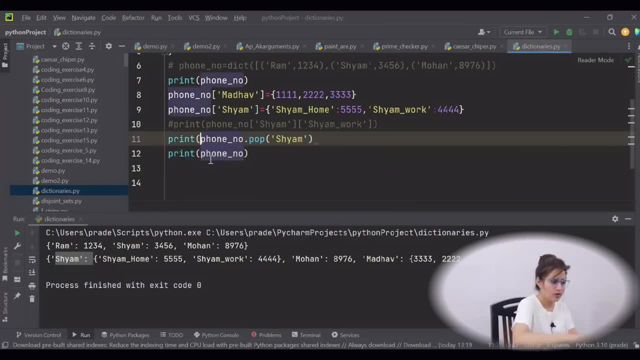 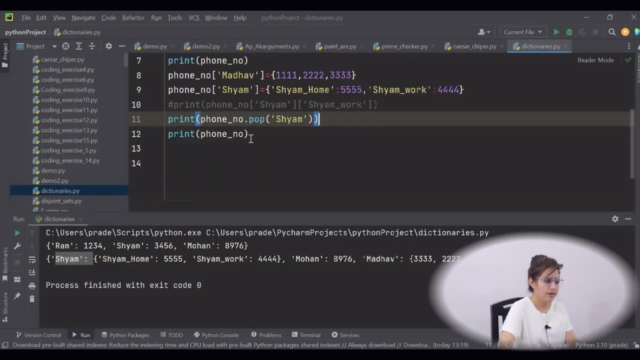 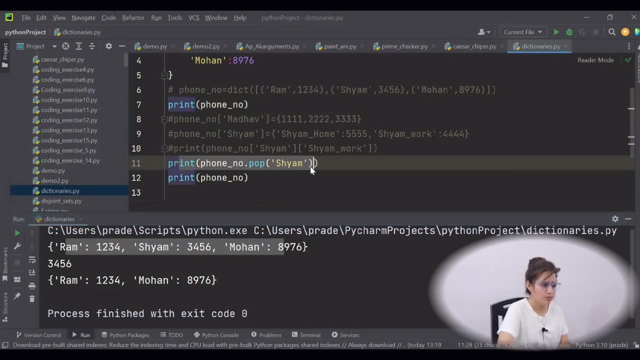 that value. So if you want to print what this pop will return, you can print that thing also, and after that we are going to print phone number, Right, Thank you? Thank you. So first is RAM, Shan and Mohan, then this pop. it will return the value corresponding. 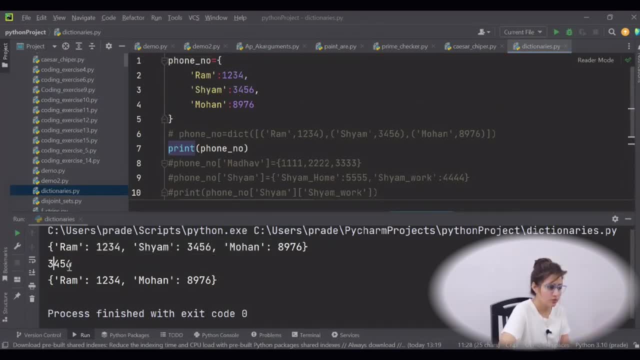 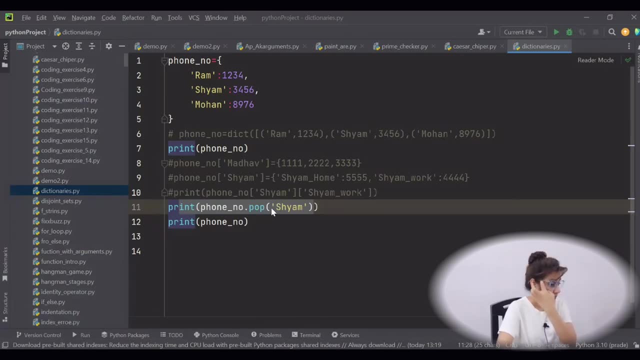 to this key, Shan. So corresponding to Shan, we are having 3456, 3456.. And then after that it will print RAM and Mohan, no, Shan. So using pop also, you can delete a particular item and we have one more function: pop item. 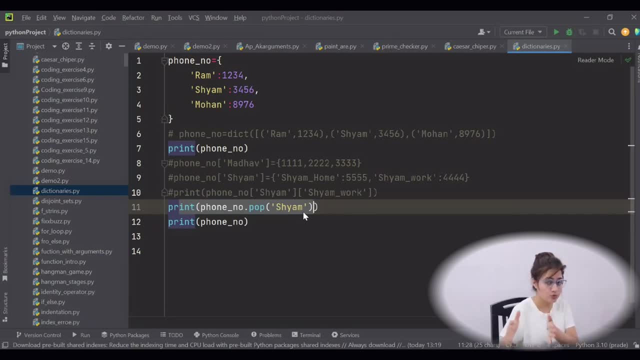 that will delete the last item added, the last one Since Python 3.7 version. this is the case, But we can delete that item effectively, I believe. So we are going to delete that. So the last item added the last one Since. 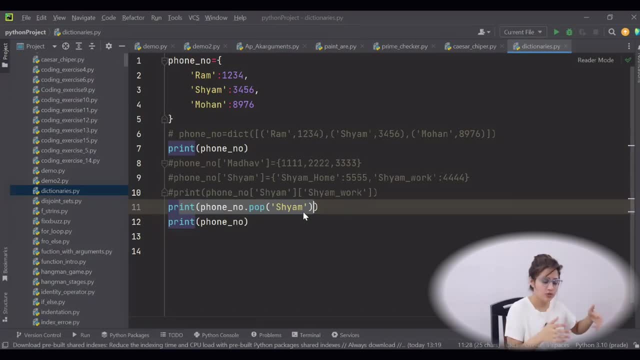 Python 3.7 version. this is the case, But we are going to show you how to delete the. But before that version, in 3.6 version and earlier version, pop item was used to delete any random item. any random item it deletes, right. 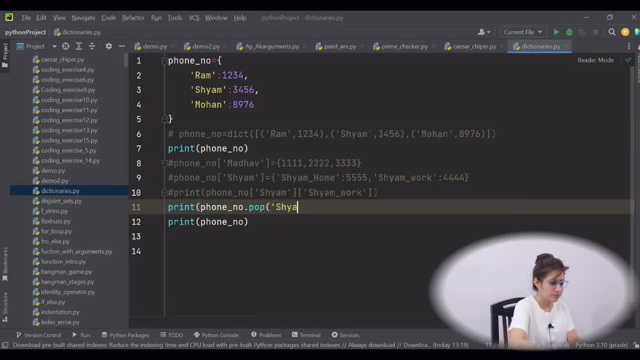 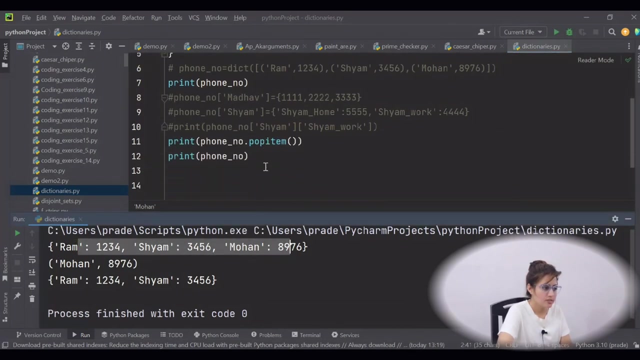 Now, if I use here pop item, so same phone number, name of the dictionary dot pop item. see, we are having pop and pop item too. pop item, right. So it will delete the last one. last one added is Mohan, So let us run this and see: first is this, then, whatever it will delete, it will return that. 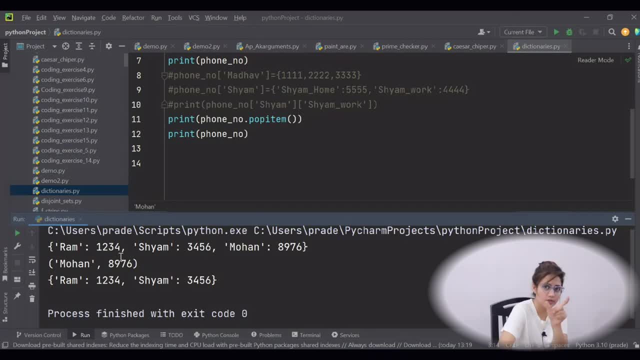 key and value both. So Mohan and this, this item. it will return that item, but pop will return only the value and after that Ram and Shyam. okay, So this is pop item One we have clear. clear will delete all the items from this. 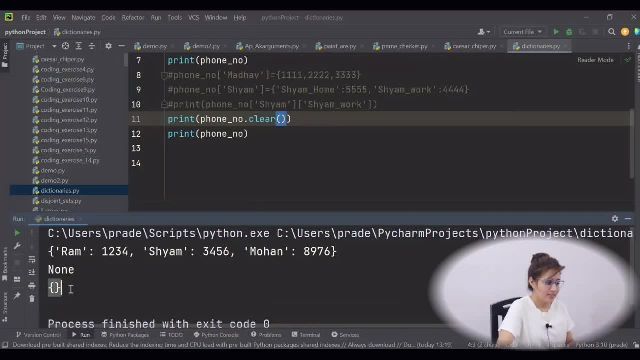 Dictionary. let us run this. see, it is none right And it will return n nothing, So let us just remove this. it will not return anything, so we are not printing anything, So let us run this again. See, first dictionary was this and then, after clear method, it is empty. nothing is there. 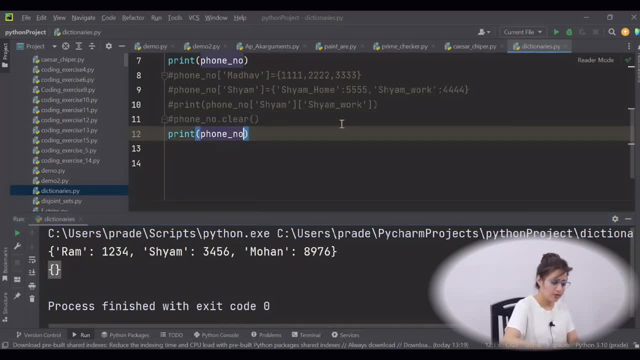 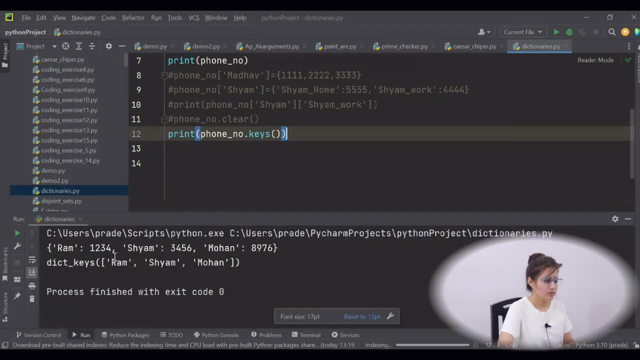 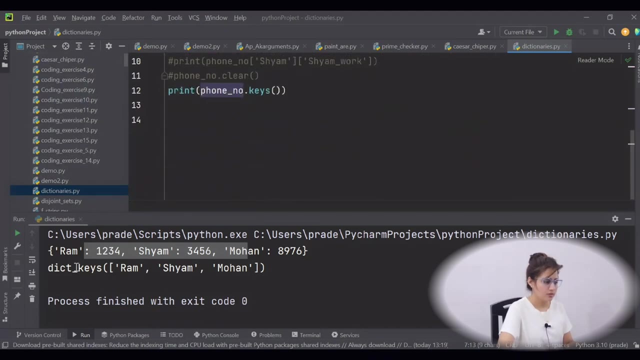 okay, If you want to access only keys. so we have also a built-in method. name of the dictionary: dot keys. Okay, Let us run this and see. first is the dictionary, because we have printed here phone number right, Then only keys. dict. underscore keys are: Ram Shyam Mohan. 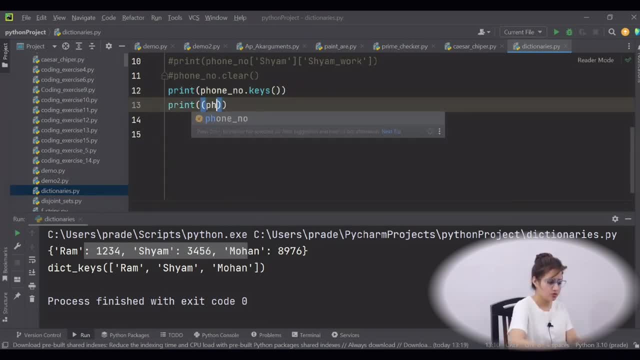 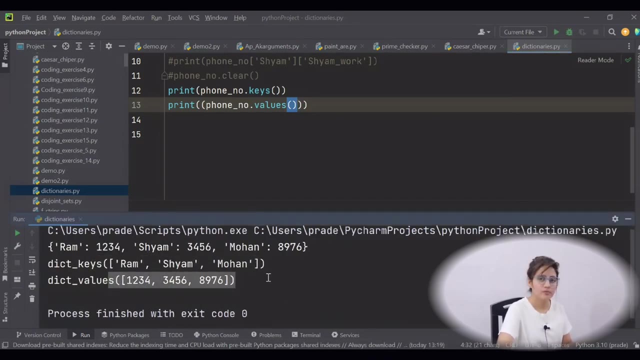 If you want to print only values, for that also we have a function built-in function: dot values. okay, Now let us run this: See dict. underscore keys are: Ram Shyam Mohan. Okay, Dict keys, dict values: right. 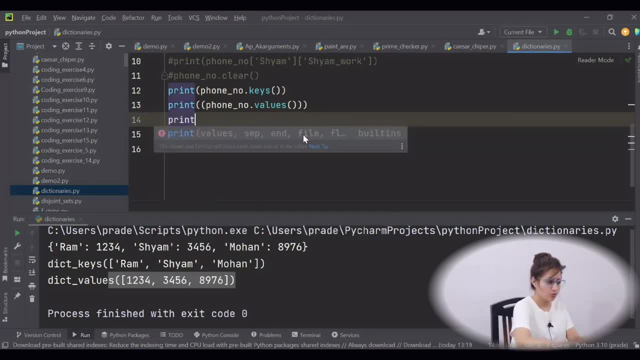 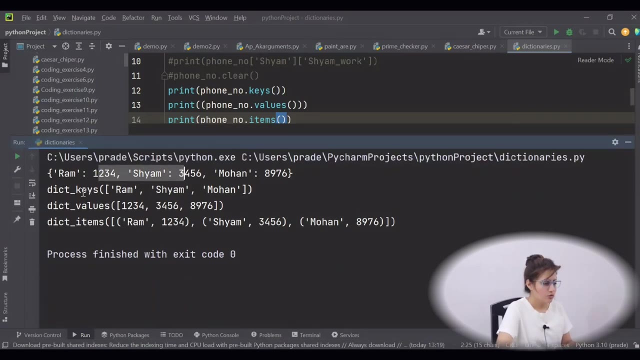 We have one more function that is item. So if you want to print that also what it will return. Let us see Phone number dot. this function is very important. items. let us run this See: first was this, then keys, then values. we have printed, then dot items. so item will. 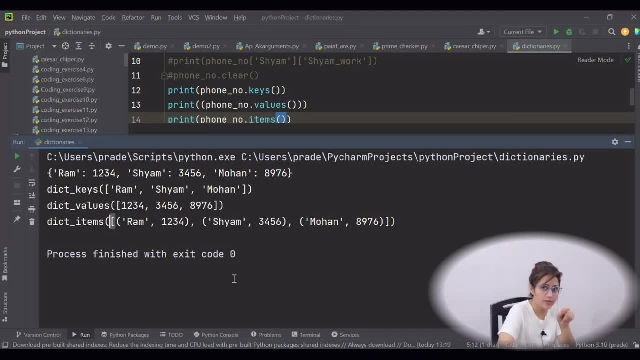 print list: See Square brackets. Square bracket is there, So it is a list List of all the items, but in the form of tuples, See. this is a tuple: Ram 1,, 2,, 3, 4 in round brackets. 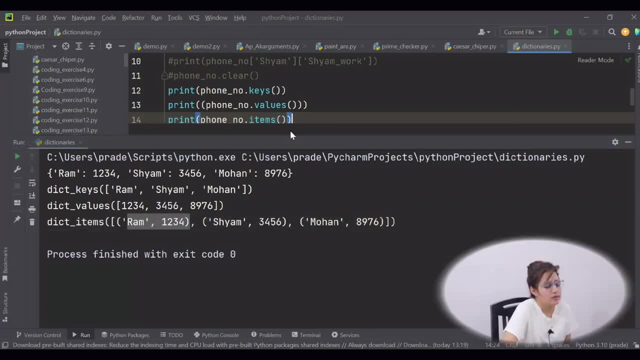 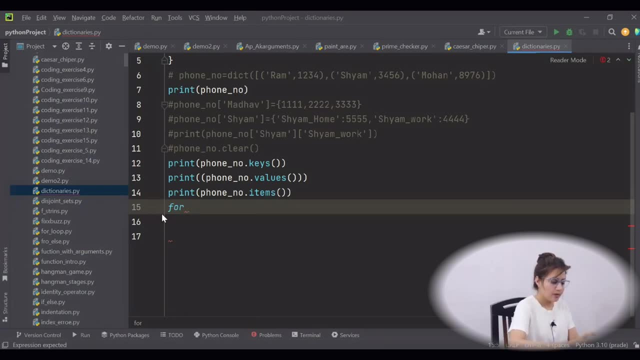 So one tuple, two tuple, three tuple, In for loop. also we can loop through this dictionary using for. so for if I write for any, suppose simple, any variable, I am taking I in phone number And I am just printing: Okay, Okay. 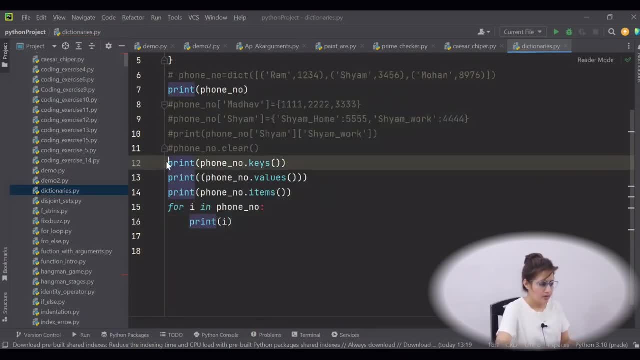 So this is printing I. What do you think What it will print? Let us just comment out these lines For I in phone number and print I- What do you think what it will print? Let us see Only the keys Ram, Shyam and Mohan. 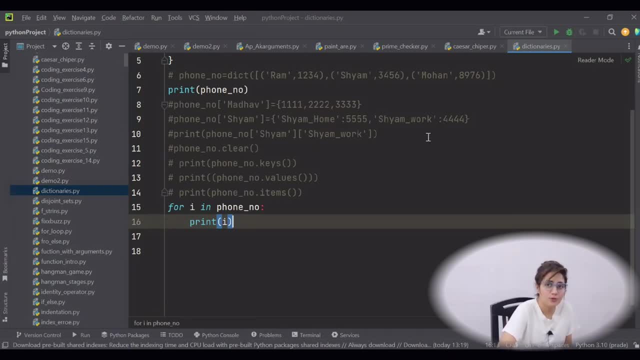 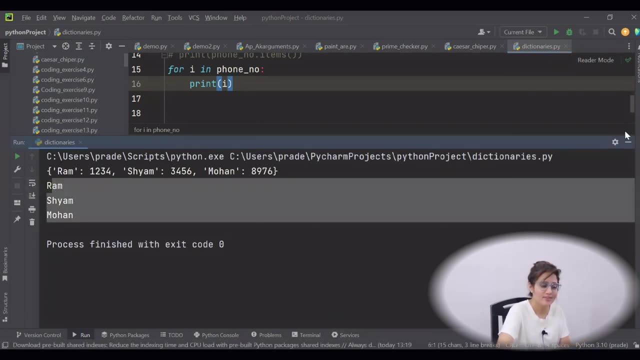 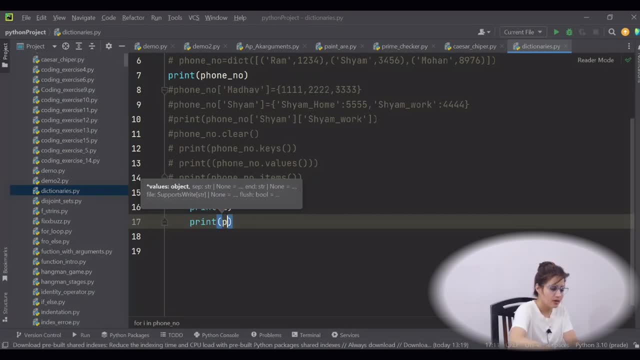 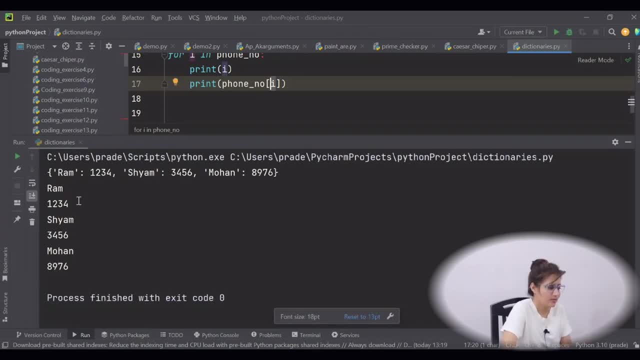 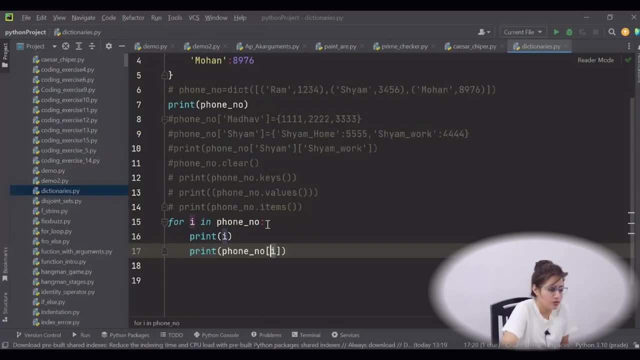 Because this is how you can access the values: by passing the key. Let us run this Now: see Ram, then value Khan, then value, then Mohan, then value Okay, And in for loop also. we can use that item functions. so phone dot items. 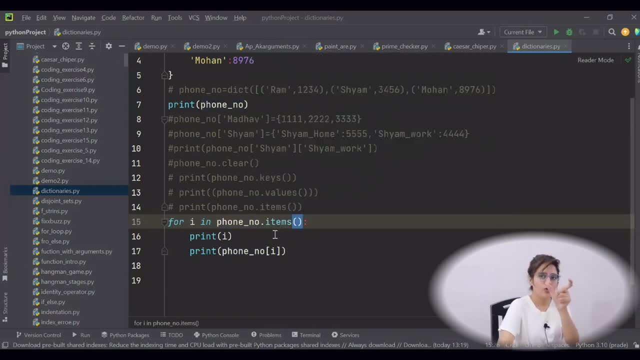 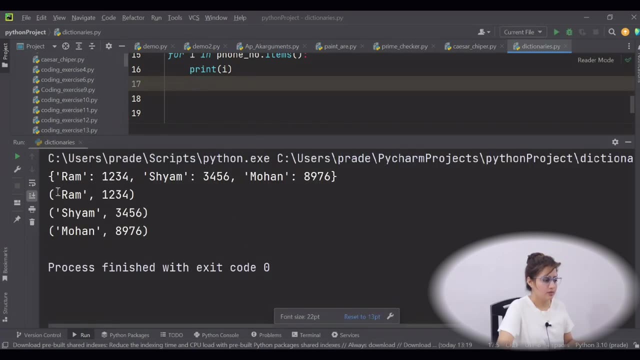 So it will print key and value pair Right. So in this case, if I print this, I What it will print? print c: All these items in tuple, but individual. first is this, second is this, third is this, or you can say it will return a list of tuple pairs. 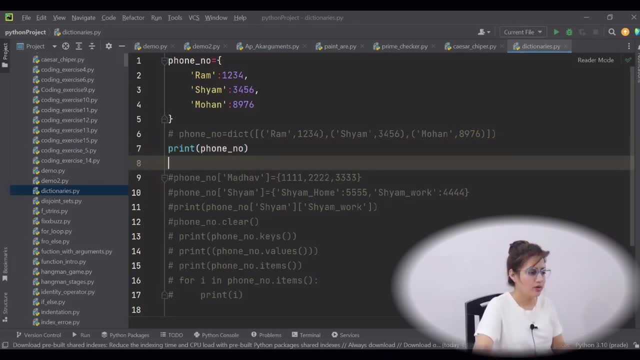 And if you want to copy this dictionary to another one, for that also we have. we have a function inbuilt, function copy. So what you can do, The name of second dictionary, suppose phone number 2, equal to this dictionary, phone number dot. we have a function c copy. 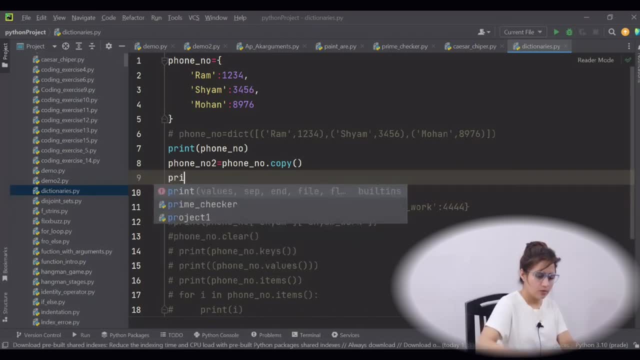 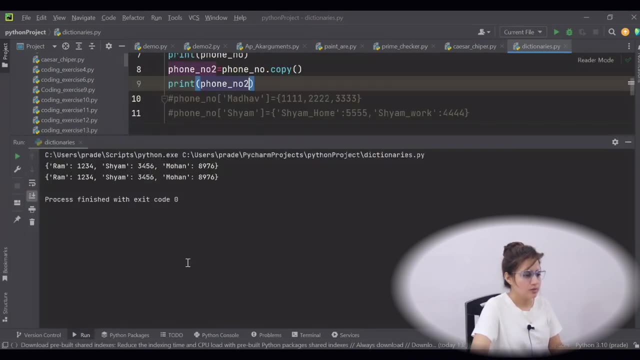 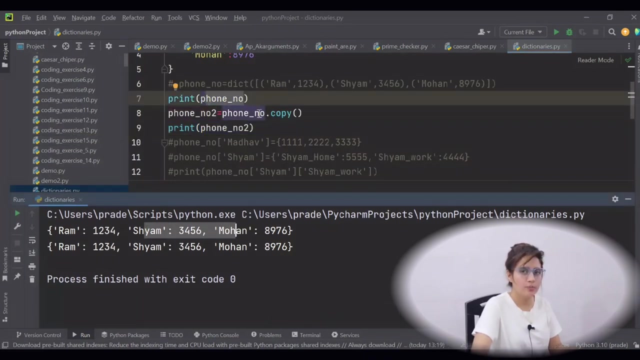 And after that just print phone number 2,. let us run this. So see: first print statement is phone number. this phone number I am printing, then we are just copying this and then I am printing phone number 2.. So same you will get. So if you want to copy as it is content. 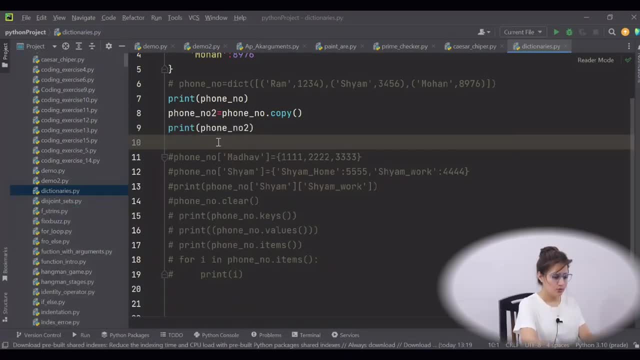 you can do that thing also. And if you want to find out length of a dictionary, for that also we have a function length function. So you can just print using length function, len and the name of that dictionary. Let us just comment out these two lines. let us run. 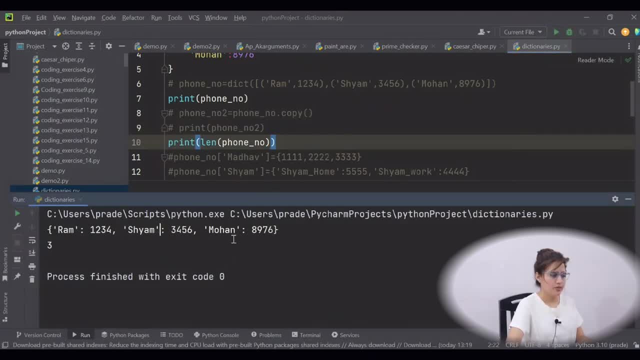 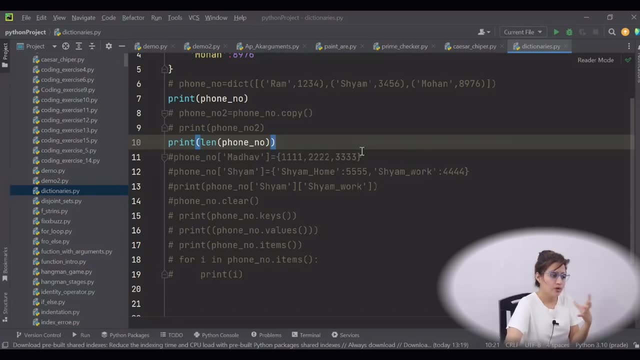 this See: length is 3, 1,, 2, 3 item we are having, So length is 3.. So this is. there are many built in functions also. You can just check out, you can just google that functions and you can try to use those. 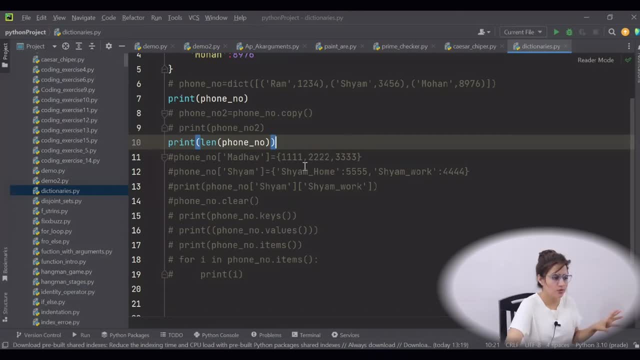 functions? What are you know generally, whatever function we will use, that I have told you. but there are many functions in built function. You can just try out many functions and if you are not getting anything you can just ask me in comment section, like how this function. 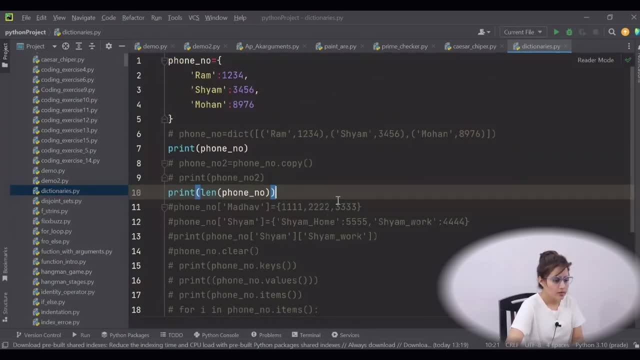 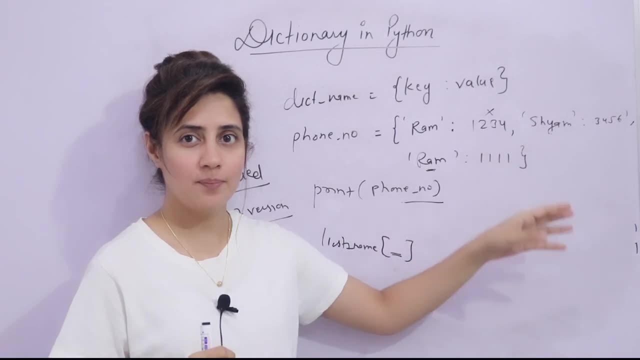 is working right. So that is all about, I think, dictionaries. So I hope you got what are dictionaries in python, how these are different from list, set and tuple, some properties, some built in function in dictionaries, The syntax and how we can use, when we should use, dictionaries in python or in our program. 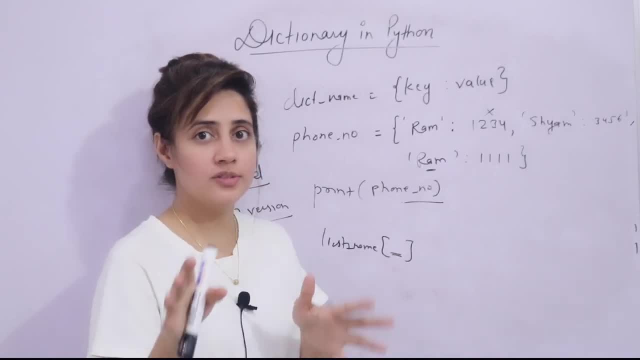 right, So now I will see you in the next video. In the next video, we will see one coding exercise based on dictionaries. ok, Till then, bye, bye, Take care.